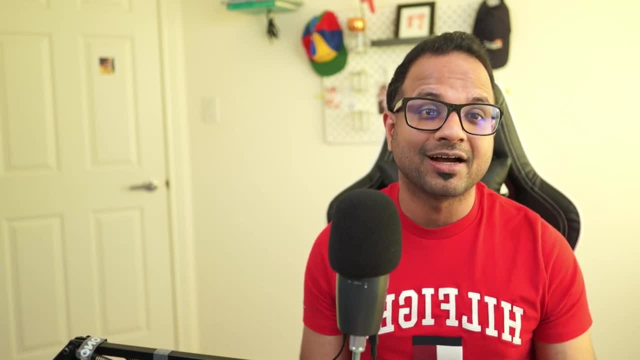 have completed the challenge successfully. For those of you that are new to cloud or DevOps and couldn't complete it, do not worry. In this video, I'm going to show you a step by step process of how to achieve all these tasks, So just be with me for a few minutes. 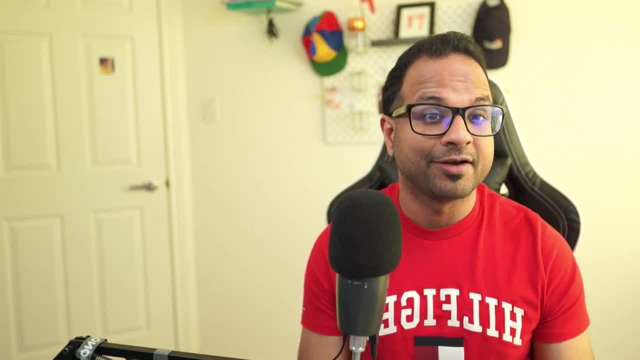 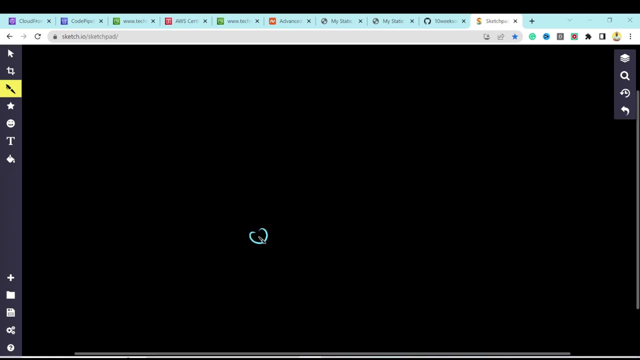 and you can pause the video whenever you feel like, and you can follow along with me. So, without any further ado, let's start the demo. All right, so this is what we will be doing. Let's say you have a user who wants to access your website, So that user will hit your DNS. 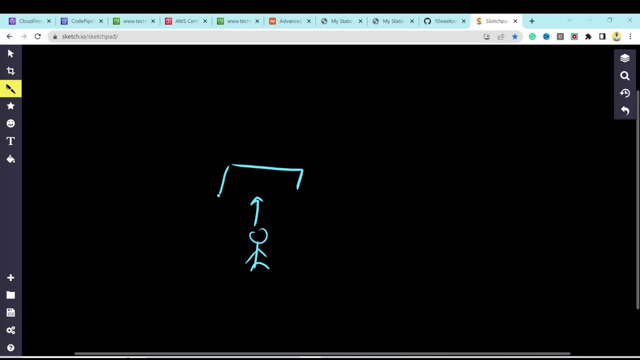 in the web browser and there'll be a DNS service that will be accessed on the back end. In my case it is Namecheap, So this is the DNS service that I'm using. Then that DNS service will have a CNAME record, which will redirect the DNS to your CloudFront distribution. Okay. so, just like the DNS record on the backend, you have to go through the CloudFront distribution where you want to store data like the archive, such as an email address or just the password. You can also use your ID and password that you just typed. in the end of the day I'm going to 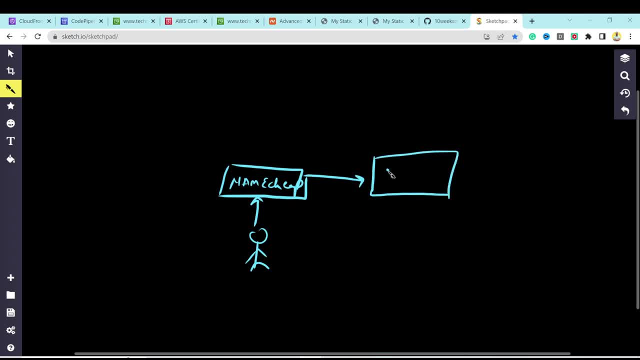 so our cloud front is a cdn service that you are using cloud front and then the cloud front will be serving the static content from the s3 bucket. so this is your s3 bucket that has your indexhtml, errorhtml, all those static content and images, videos, etc. 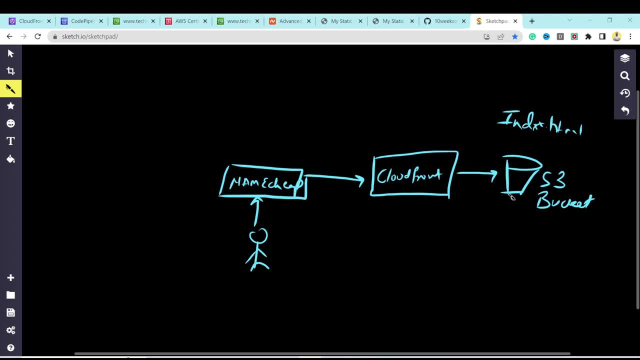 and this s3 bucket will be accessed only from the cloud front using oai origin access identity, which is a secure method to access the bucket, and user cannot directly access the s3 bucket. this is not permitted and this is not a secure practice, and we will also be using acm in front. 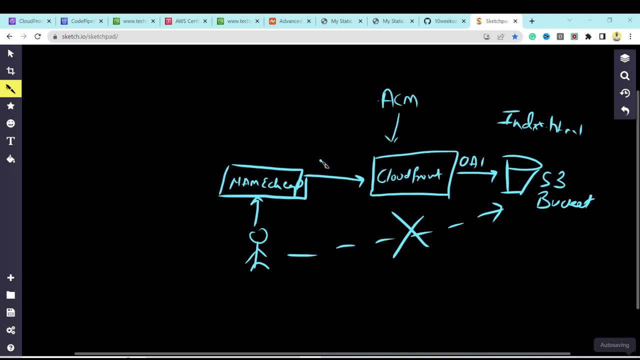 of cloud front to make this connection secure so that user will be able to access the website over sdps. so the services that we are using over here is a dns service, such as namecheap route 53 or godaddy content delivery network, such as cloud front certificate manager, such as acm s3 bucket to host the website content, and so on. 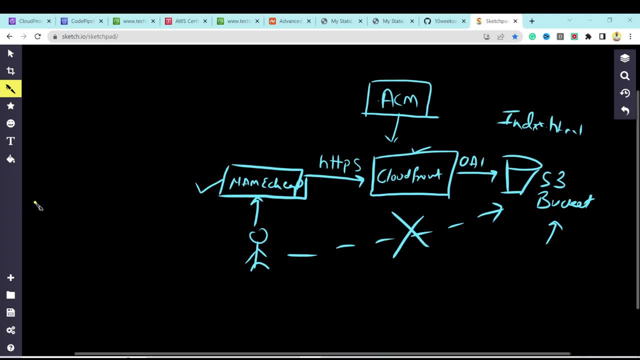 now, once these steps are completed, you will be able to access the website and you will be able to access the s3 bucket. the next step would be to automate the complete process. that means whenever a developer checks in the code, it should be automatically deployed to s3 bucket. so to do that, let's say the code is: 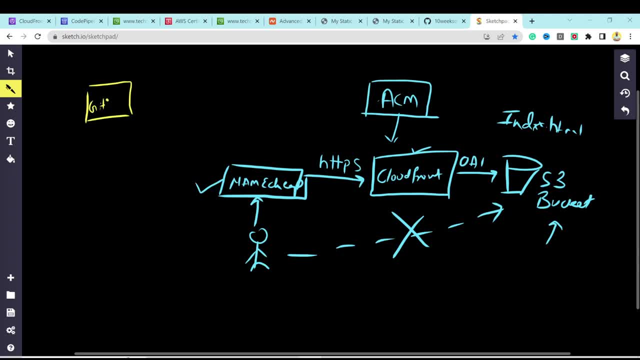 hosted on a github repository over here, github and your developer. whenever the developer do the code check-in, it should automatically trigger a code pipeline which resides inside aws, and this code pipeline will then deploy the files to s3 bucket over here. let's see how it's done. 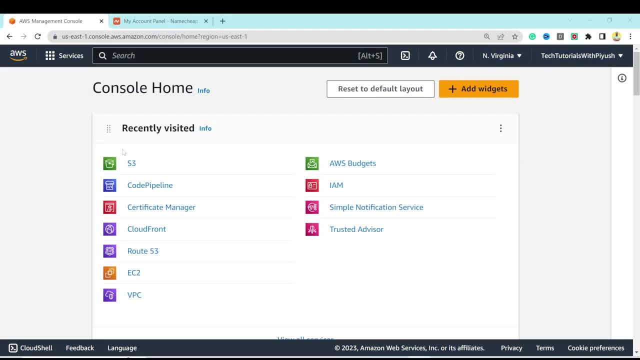 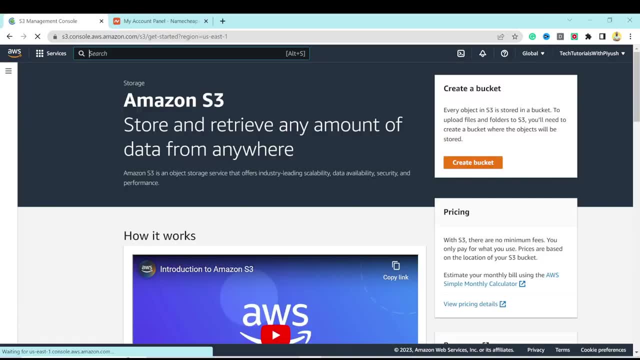 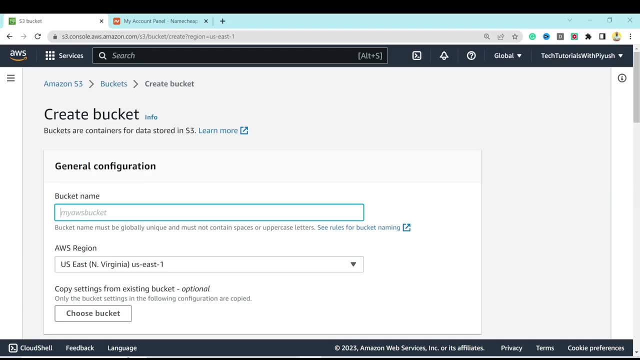 so i have logged into my aws console and i'm gonna go ahead and create an s3 bucket. i can click over here and then click over here, which says create bucket. now over here, give it a name, make sure the name is same as your s3 bucket, and then click on create bucket and then click on. 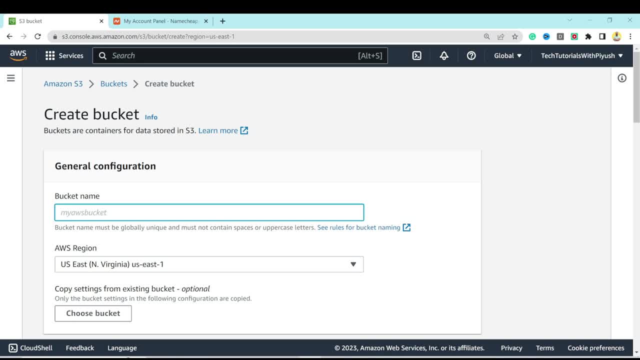 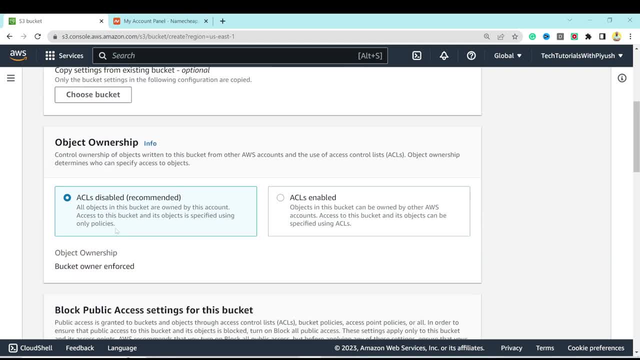 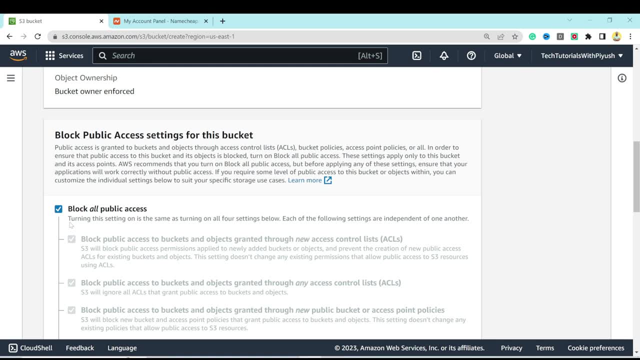 and acl is disabled, let's keep the default settings. and here it says: block all public access. so this is really important: do not uncheck this, because that will make your bucket publicly accessible, which is what we don't want. to do. that then you must be thinking: how do 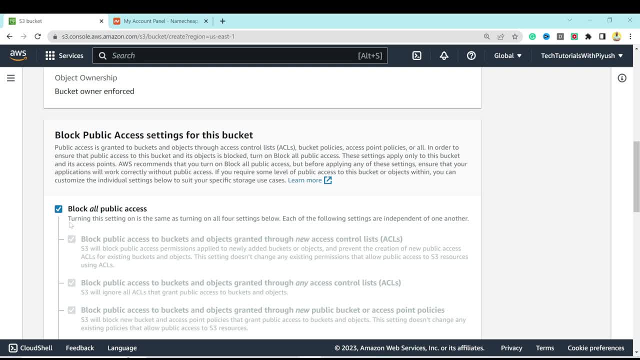 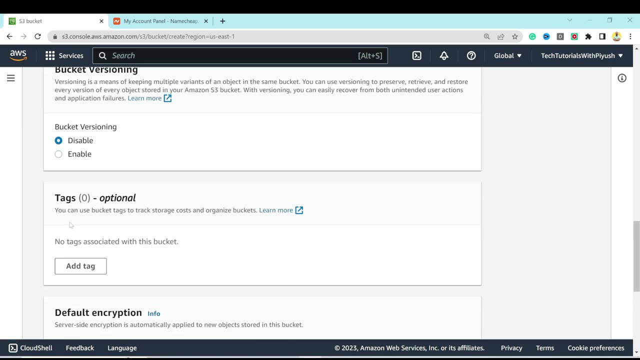 we serve the content from s3. if the bucket is not public, well, we will be serving it through cloud front. i'm gonna show you later on, after this step, but make sure this step is the default setting. that means public access is blocked on this bucket. right and scroll down and keep. 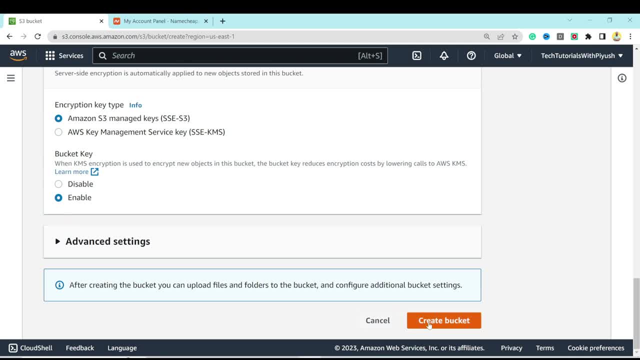 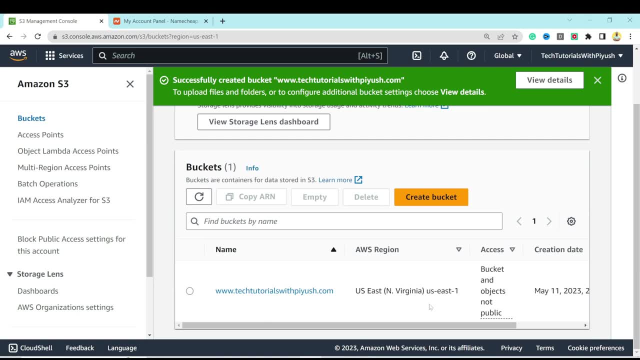 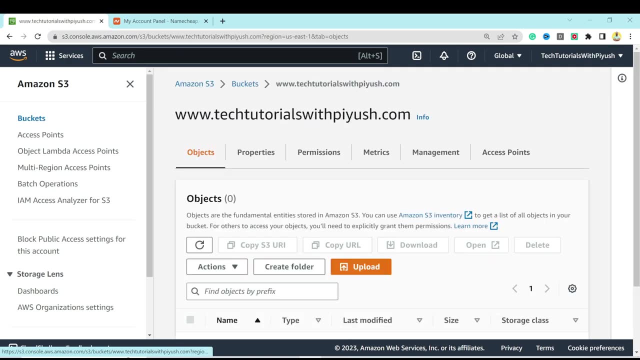 everything- the default settings- and hit create bucket. so it will take even fraction of setting and your bucket will be created and it says the bucket and objects are not public, which is what we want. now go inside the bucket. click over here and go to properties, the second tab, over here. 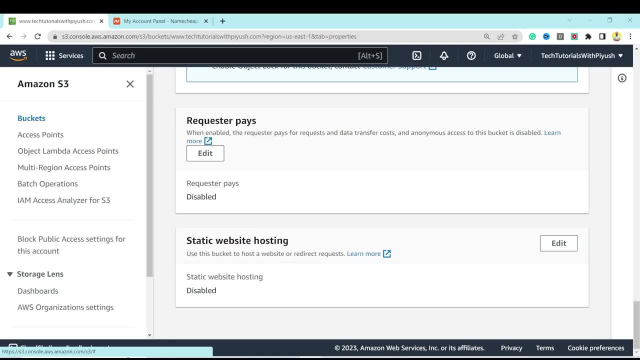 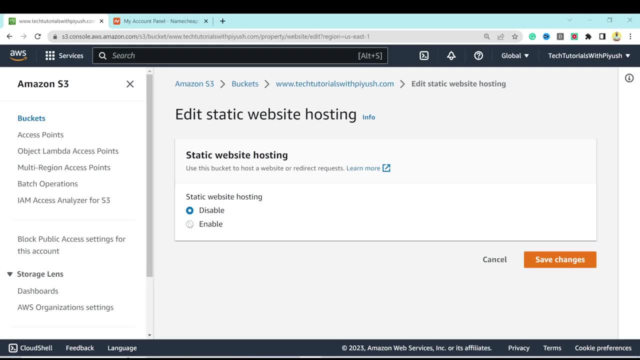 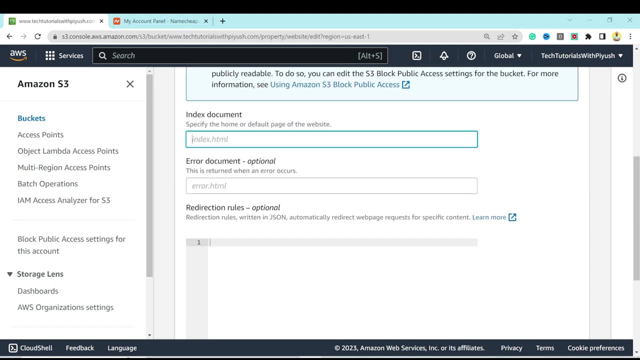 now scroll down to the very last section where it says static website hosting. go to the right and click on add it and then hit enable to enable hosting a static website, and then go down. enter your index document, indexhtml, and your error document, errorhtml. go down and hit save changes. 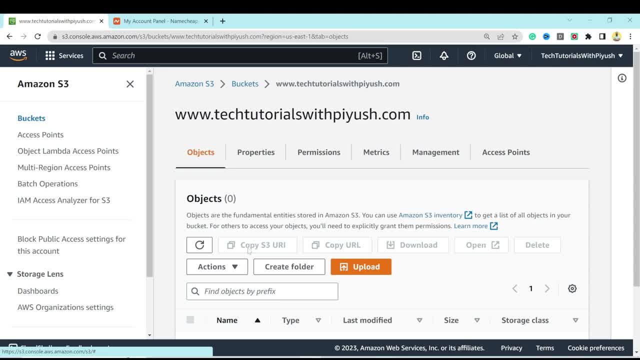 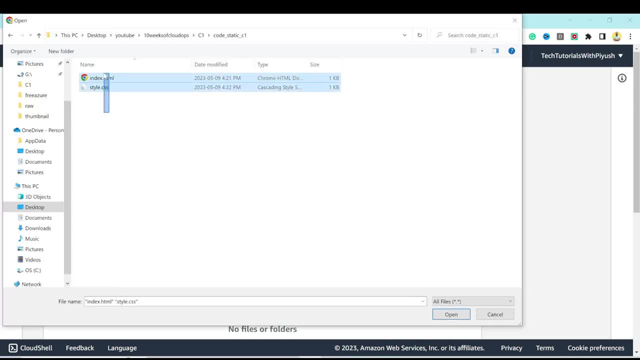 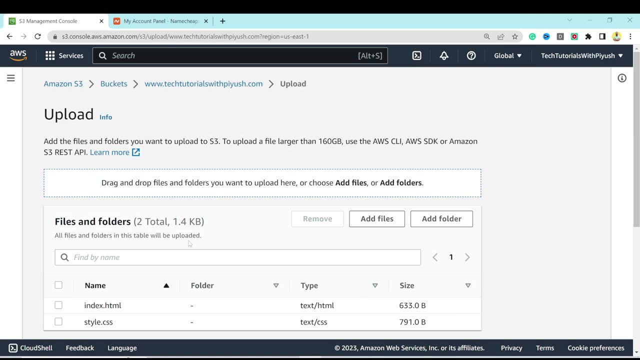 now go to object section over here and upload your static website. click upload- add files. now i have these two pages: indexhtml and stylecss. this is what i'm gonna use. so this is pretty basic website, nothing fancy. just wanted to show the other features of it, like how: 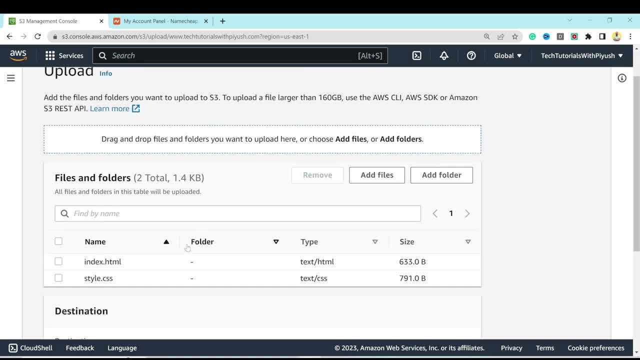 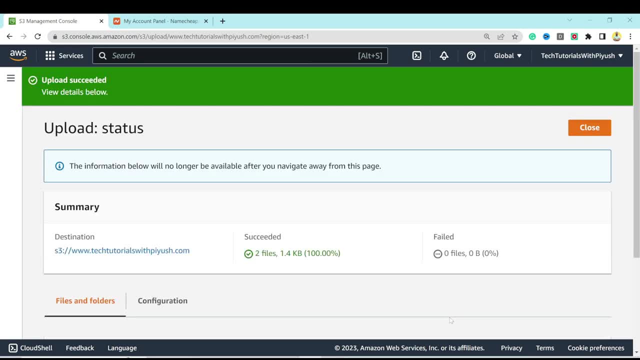 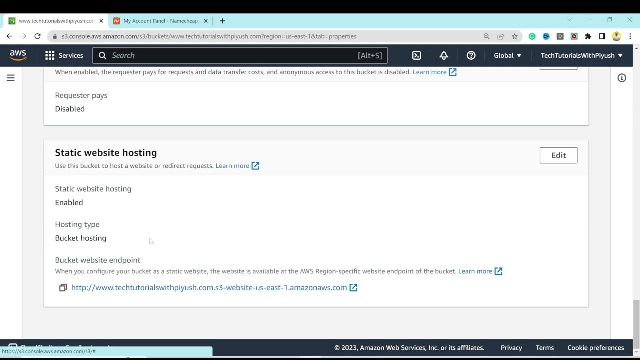 do we host it? how do we secure it? so that's why i kept it to the minimum and just scroll down, verify everything and hit upload. all right, so hit close and go to properties again. go to the last section where it says so this is your bucket endpoint. 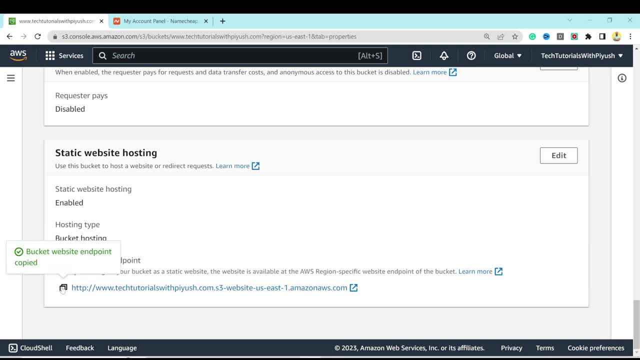 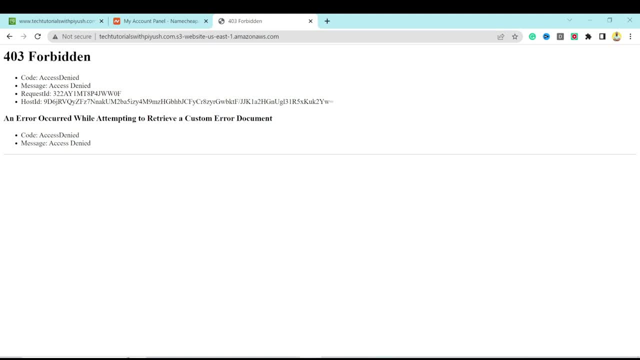 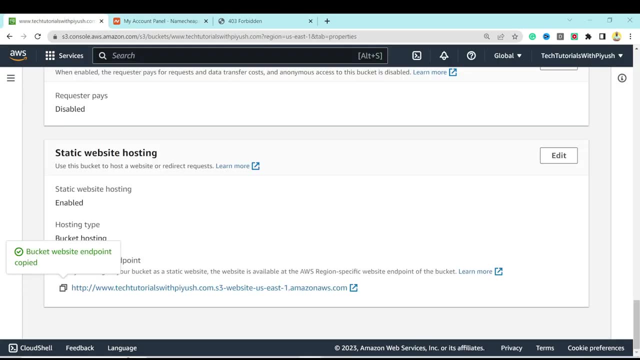 on the url where bucket will be accessible. if you hit, copy and paste it in your browser, this should show you permission denied, which is what it is right now, because we have disabled the public access. so we are good till now. now go ahead again to your aws console and 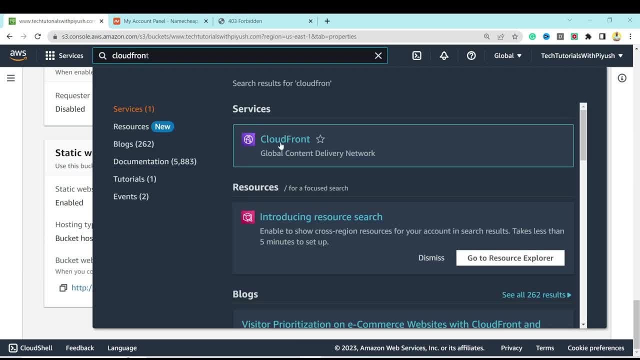 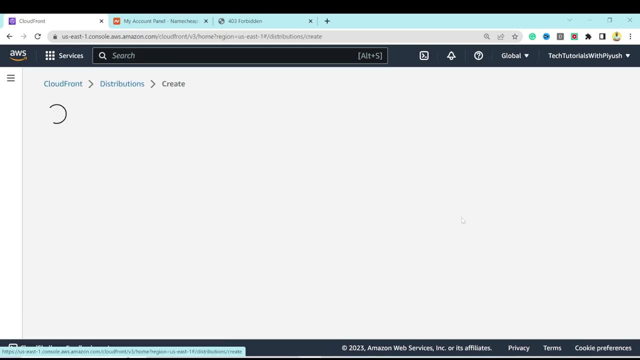 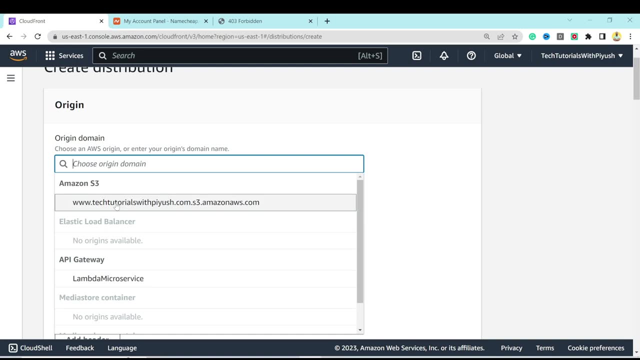 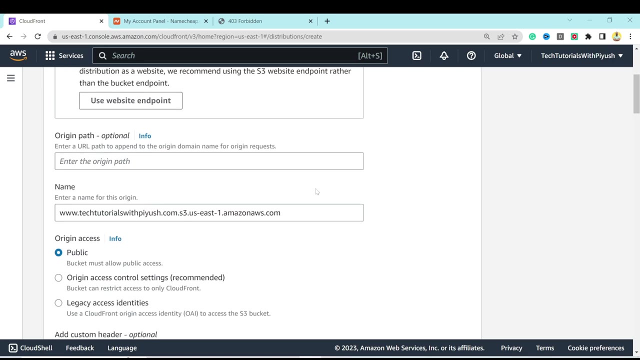 search for cloud front, because now we will be creating a cloud front origin right and create a cloud front distribution. now choose origin domain. your bucket should be auto populated over here. select your endpoint url and ignore this error warning. now this is the name of your origin, which is again auto populated with the bucket endpoint name. 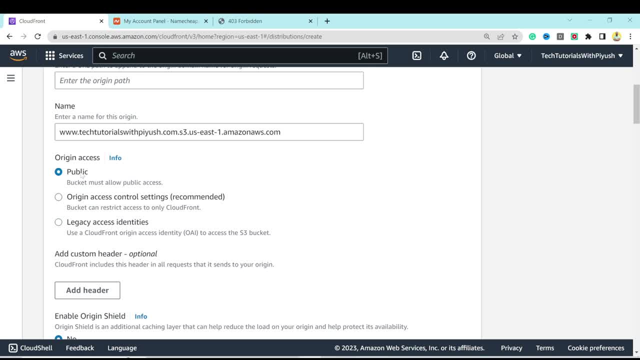 over here. your origin access is public. origin access control setting or legacy access error setting or recent access mistakes: 6000, mostly x bldir. so that this is what we need, so that we could enable the access from origin access identity right and miss tääle stumble party here on the. 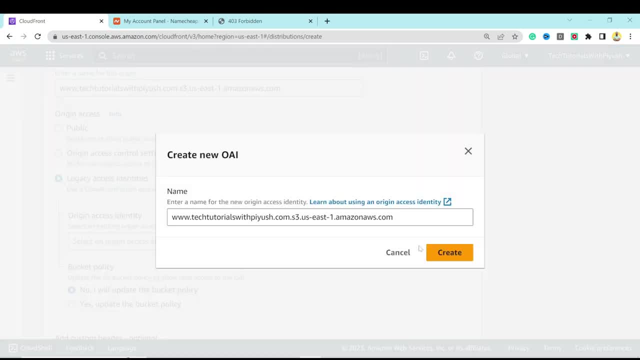 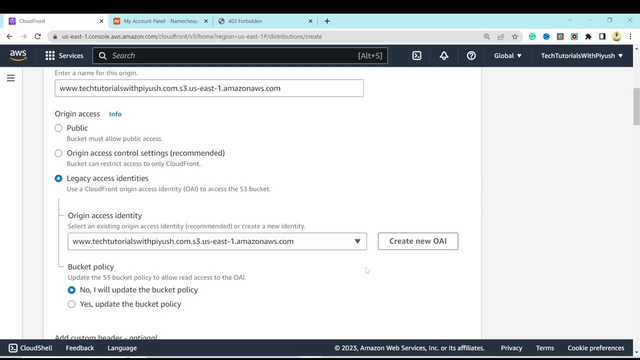 right side, which says: create new oai origin access identity and it will create a new one for you. now this identity will be kind of a user that has access to your bucket and your bucket would not be accessible from anywhere else. so this is the important step, and this is and this is why we are. 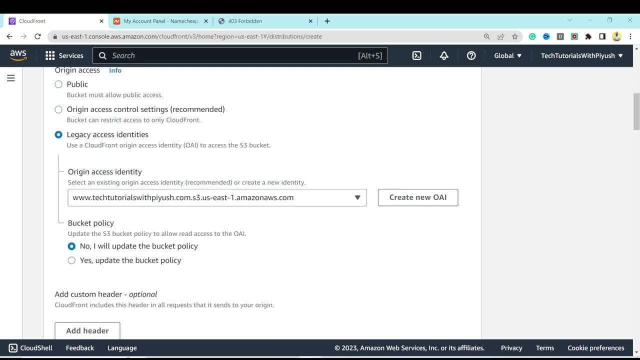 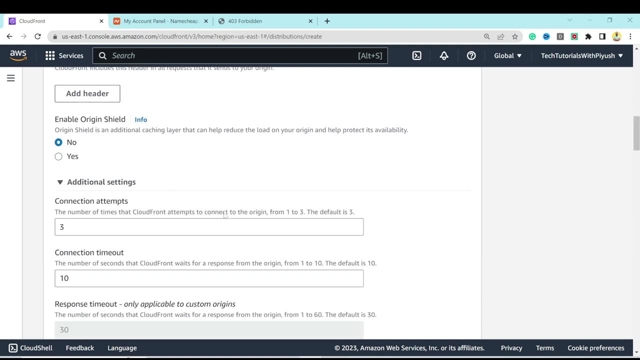 access identity. now this should be enabled in your bucket policy as well, so that your bucket would allow access to this oai. so hit over here where it says yes. update the bucket policy and scroll down. keep these settings as default. everything as default. over here, select redirect. 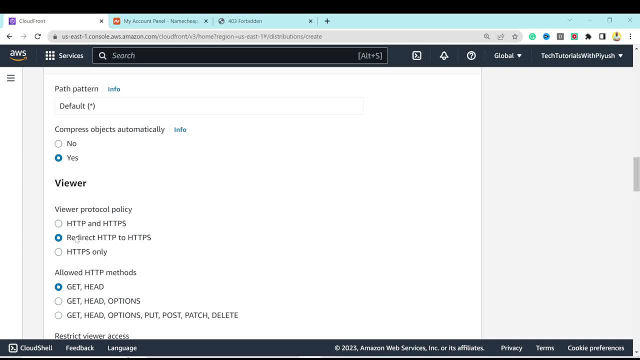 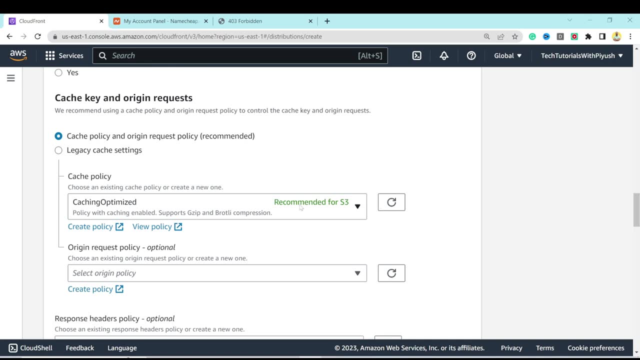 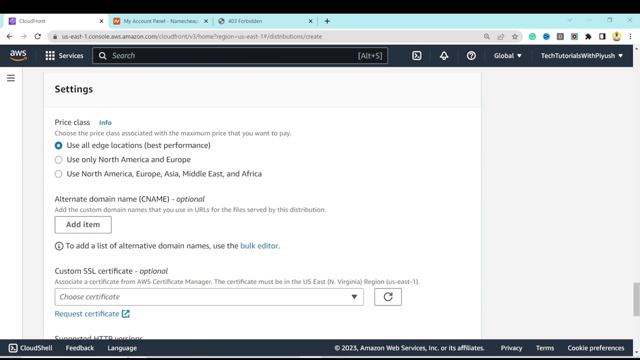 http to https, because we don't want http access. then select the http method as per your preference. let's keep it the third one for now. okay, so this is again the default settings. caching optimize, which is recommended for s3. let's keep it that way and go down. 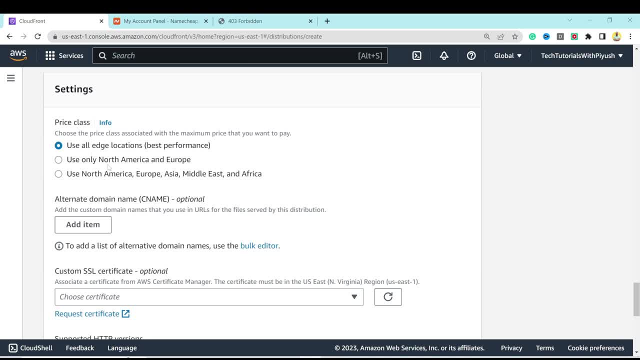 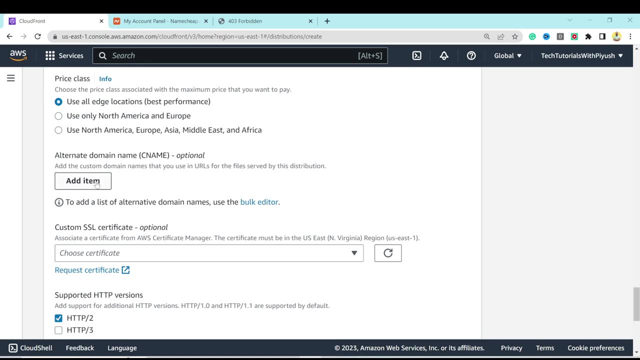 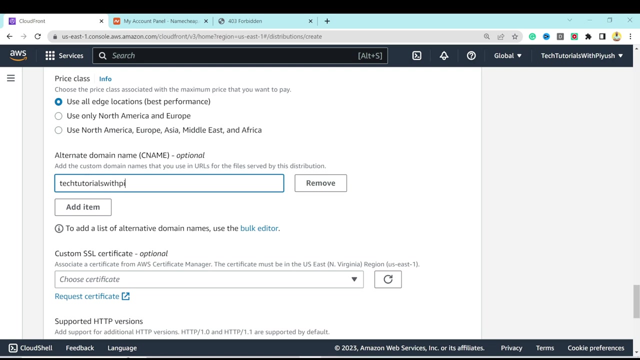 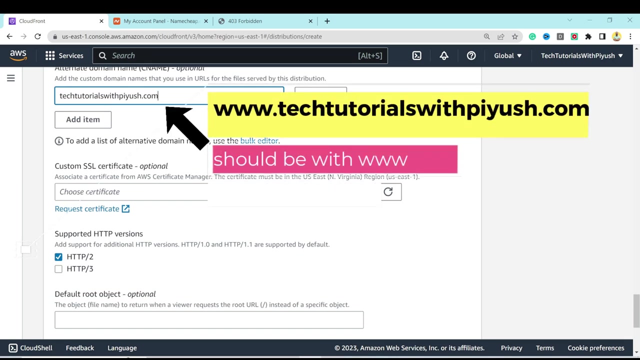 okay. now it says use all edge protection or only for some particular region. let's keep it default for now, because we would want our website to be accessible all over the world with the lowest latency possible. let's keep it that way. add an alternate domain name. let's keep it. tutorials with fuzecom now go down and now we want our traffic to. 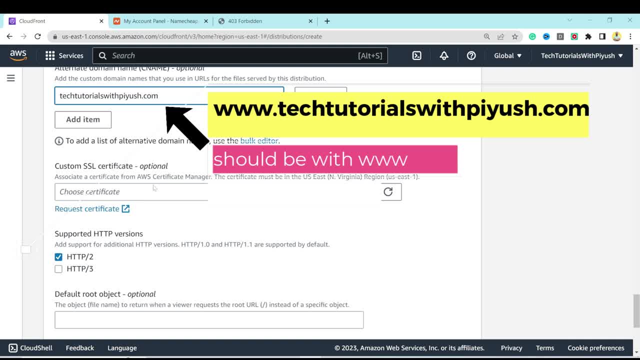 be encrypted over https. that's why we need to do that, so let's go down. and now we want our traffic to be encrypted over https. that's why we need to do that. so let's go down and to install a custom ssl certificate as well. we don't have anything created yet. 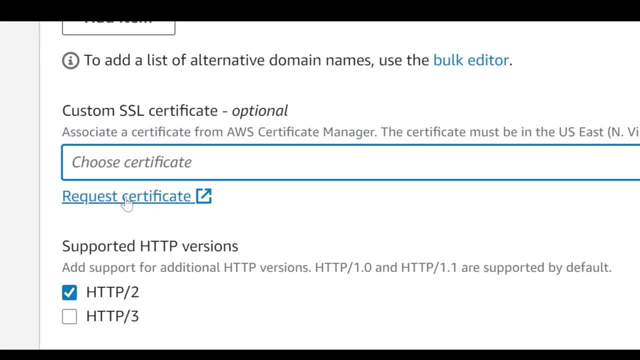 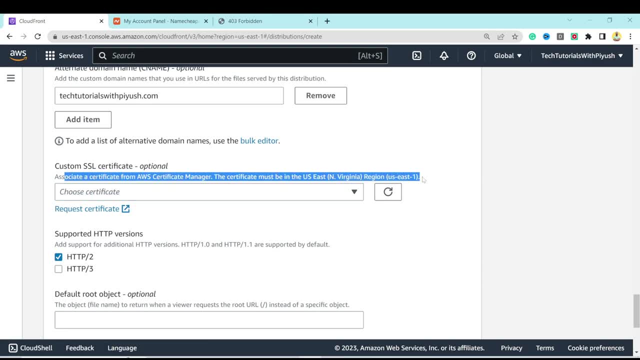 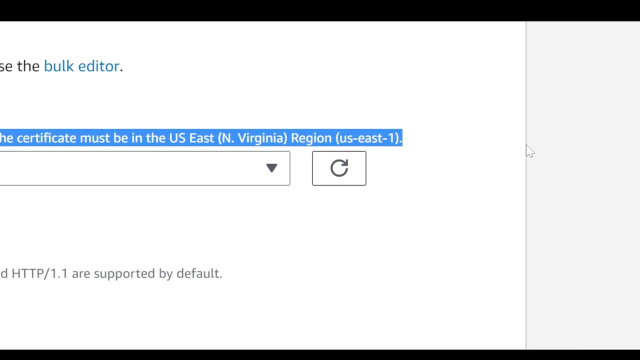 so hit over here which says request certificate, and it will open a new window. before that you must read this message over here which says the certificate must be in us east north virginia region, us east one. so that is really important, otherwise your certificate will not work. 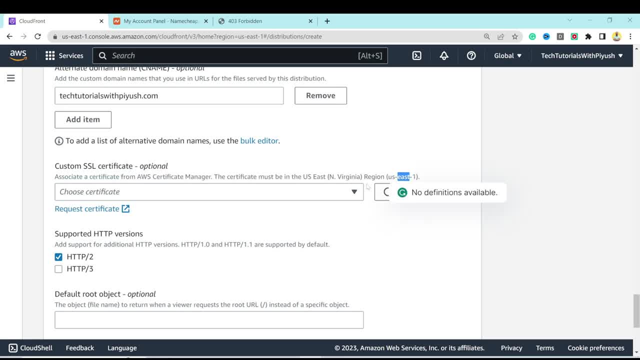 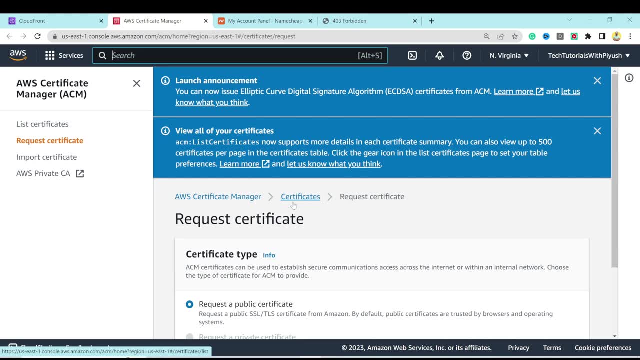 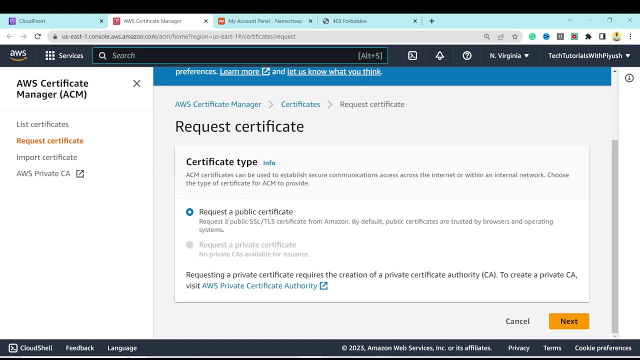 so make sure you provision your certificate in this region. only right. so let me just open this in new tab: request certificate. now there are two options: request public and private certificate. we don't have any cas available, so let's go ahead with the default option: public certificate. hit next, now enter. 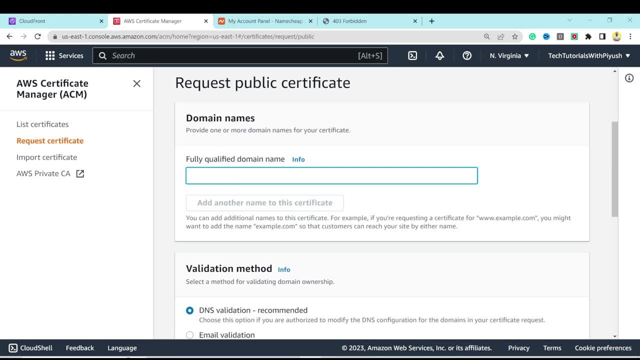 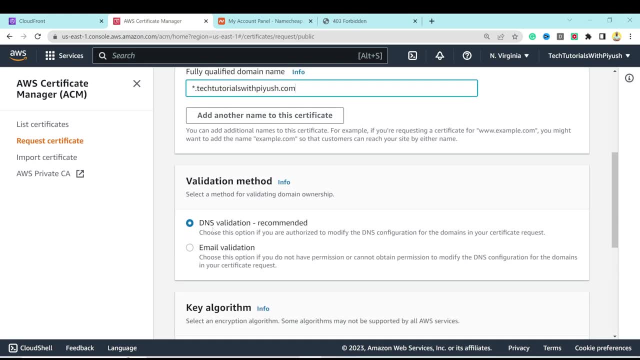 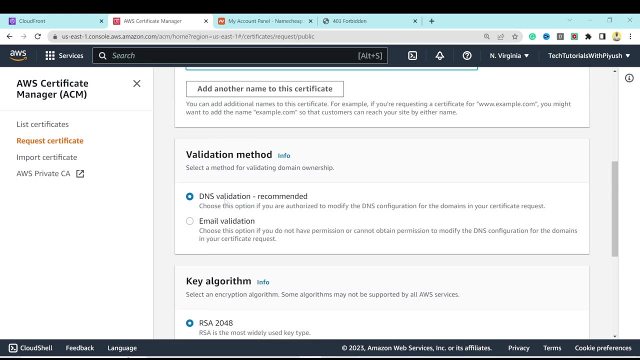 your fully qualified domain name over here. i'll just enter star dot, star dot. tech tutorials with pucecom and validation method. let's keep it dns. i'll show you how you can do the dns validation as well. so dns validation is a step that makes sure that you own the domain and you are not putting 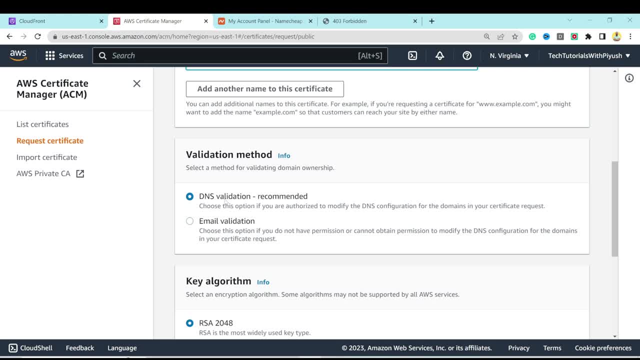 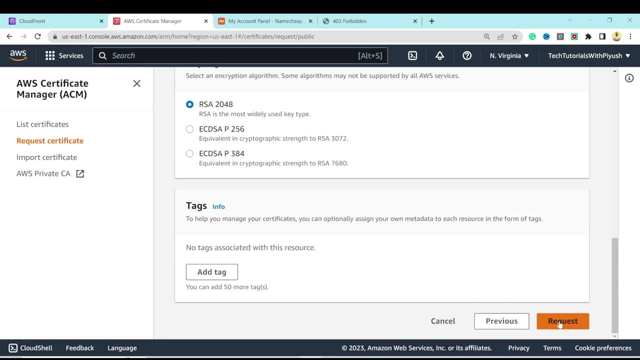 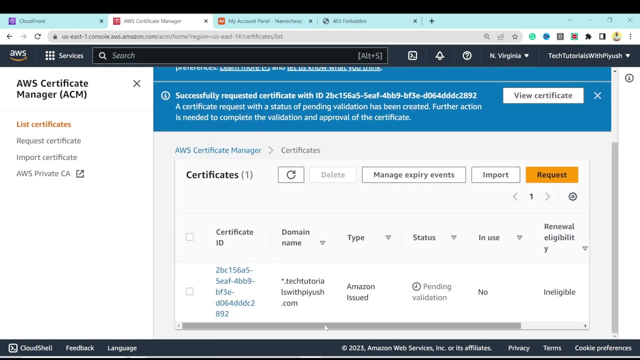 someone else's domain. so you should be authorized to modify the dns configuration to do that. i'll show you how you can do that and hit request. and you can hit request refresh over here now it will populate. it will show you pending validation because we haven't. 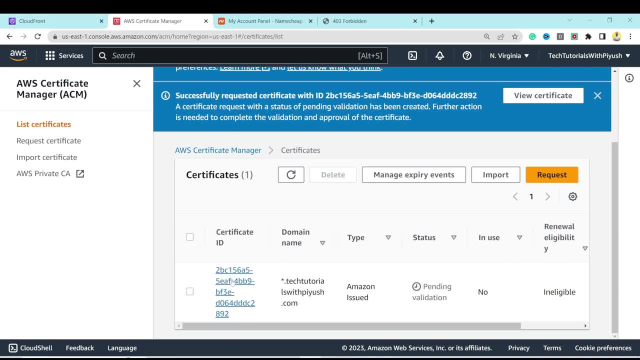 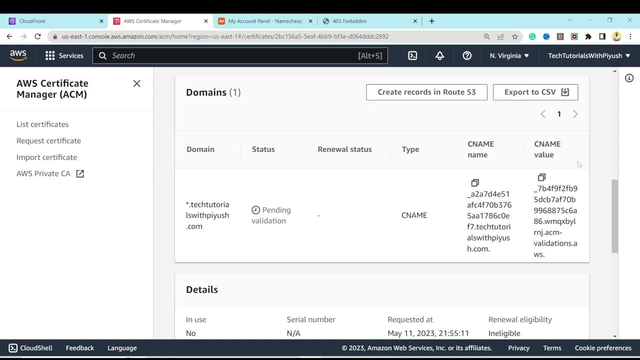 started the validation yet and if you hit over here this pending validation and it will populate a c name and c name value for you. so this c name value, using this, you can put that in your dns, whichever dns you are using, like route 53, cloudflare or namecheap godaddy, anything. 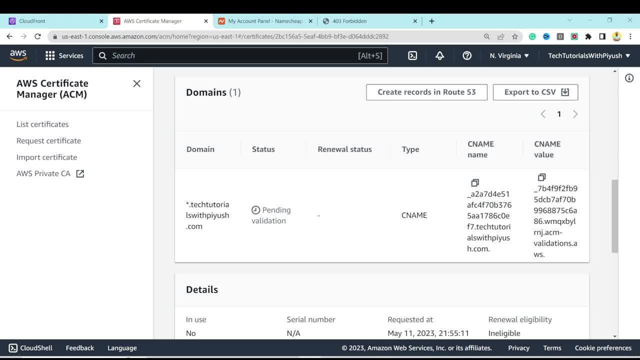 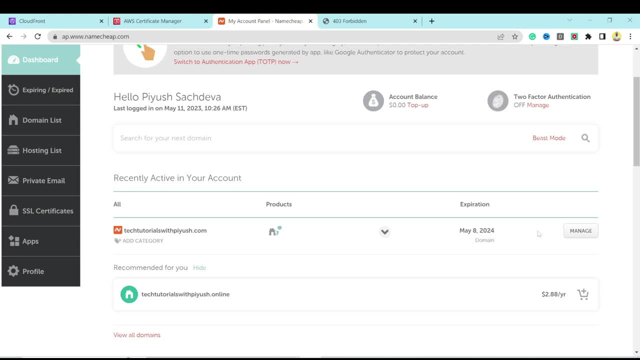 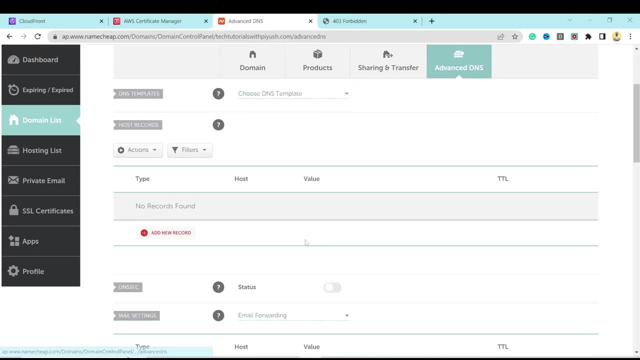 and then it will validate your dns. so as i'm using namecheap, so i'll go ahead in my namecheap window over here. this is my domain. i'll just go to the manage section. so if i go to advanced dns settings over here and scroll down where it says record, so i'm. 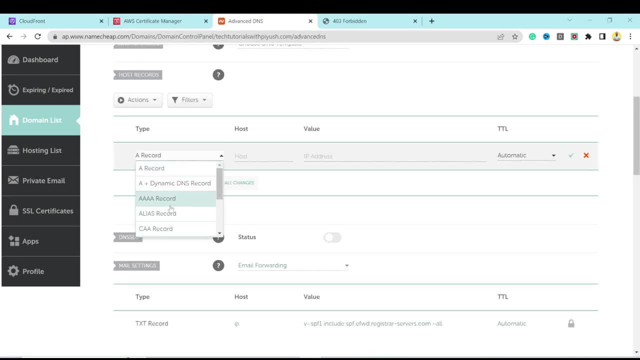 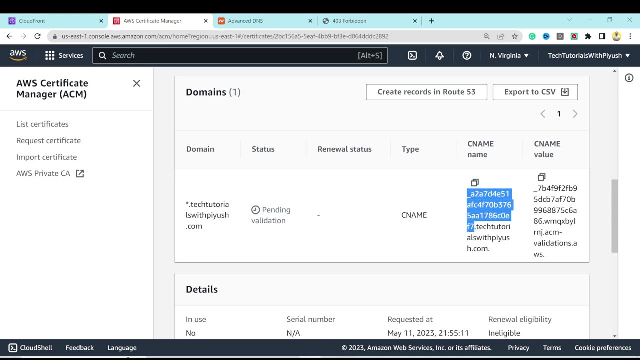 gonna add a new record and record type is cname record. now i have to put host and target to it, so the host value i'll take it from the acm itself. if you are not using route 53, make sure to copy till here, right? and because it will add the domain by itself. so just copy till here, go ahead and 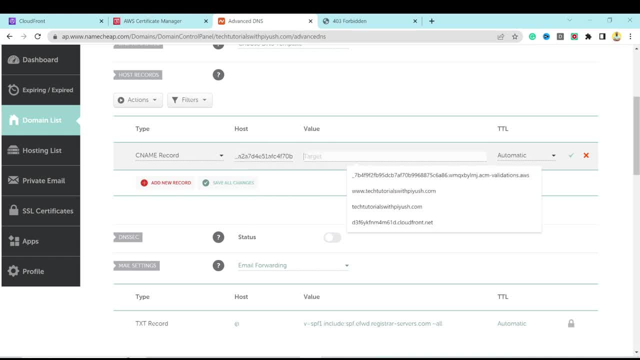 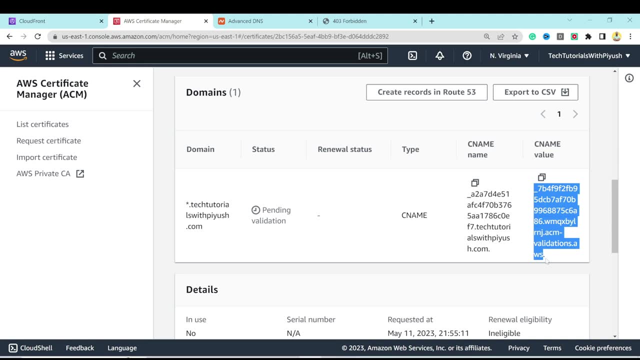 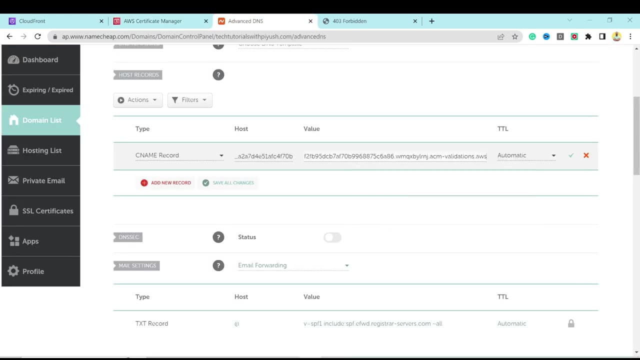 paste it as host. now i need to do the same for target value, for target as well. copy everything till aws. there is a dot at the end. please do not include that in your copy. i have copied it and now i'm gonna paste it over here and hit save changes once you do that, based on your particular 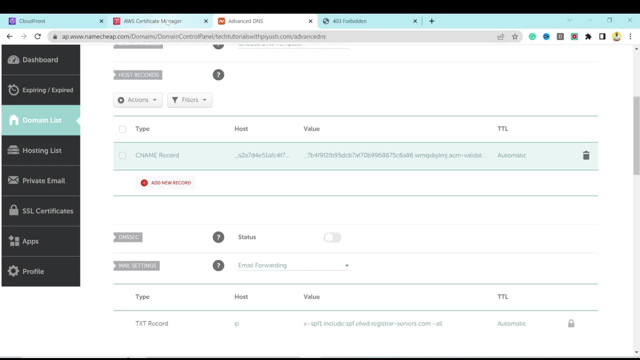 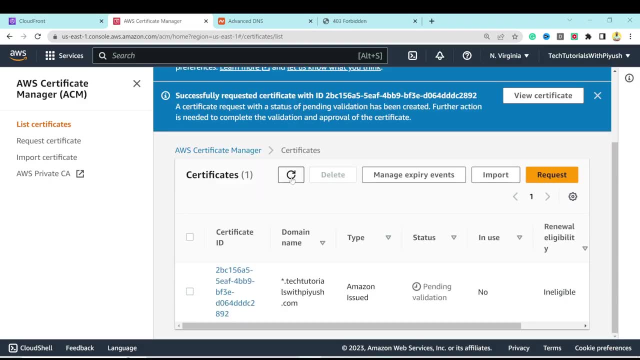 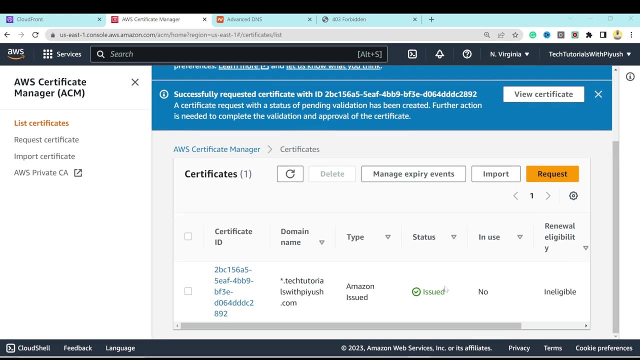 use case. it could take few seconds to few minutes to few hours, so i'll go back over here and go to certificates and hit refresh. i'm gonna pause the video and come back as soon as it is issued. all right, have waited for a couple of minutes and it's been issued. it is over here, so we are good now. 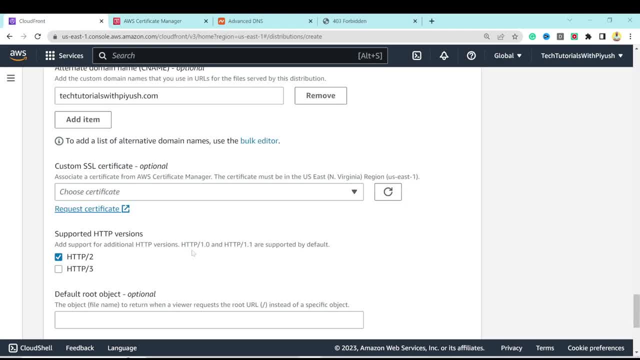 i'm gonna go back to my cloud front tab again and, uh, so this is where we were to add the custom ssl certificate. i don't see anything, so i have to hit refresh. once i do that, i see my certificate now, so i'll select it and again keep everything as default, because by default it is, it has. 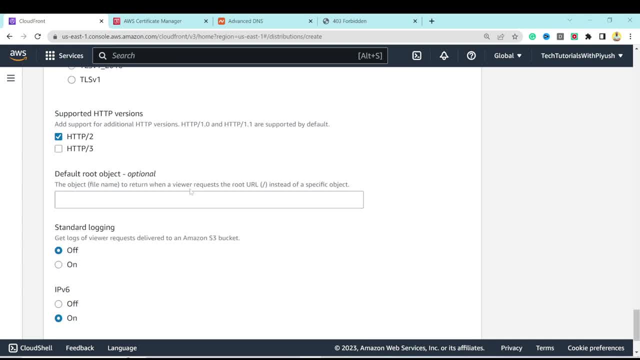 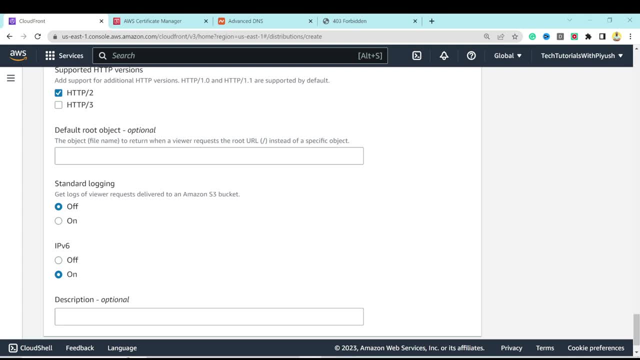 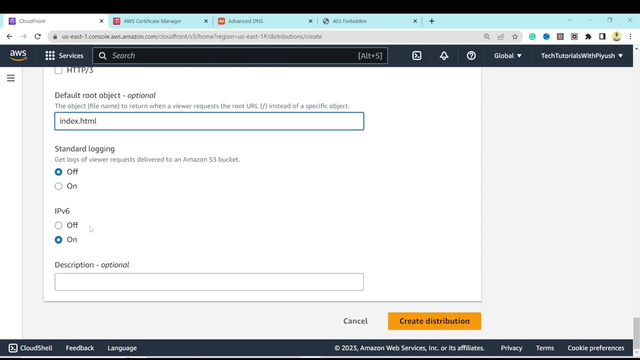 chosen the recommended settings for us, so that's good. now choose the default root object, because if you don't do that, you have to add indexhtml every time in the url, which is what we don't want to do. indexhtml standard logging off and ipv6 on. hit and create distribution. 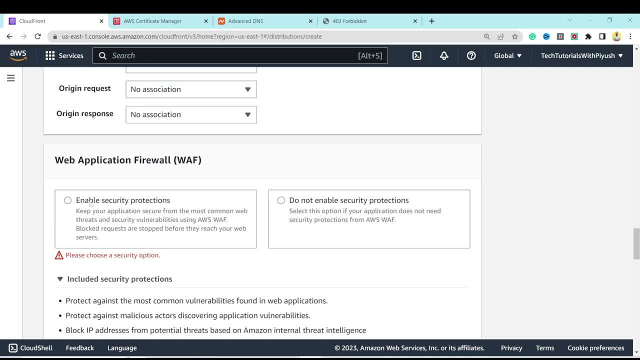 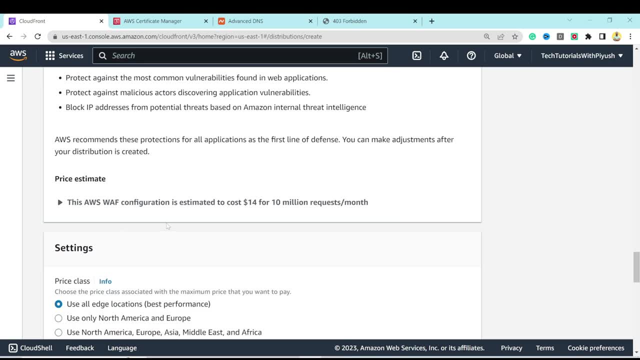 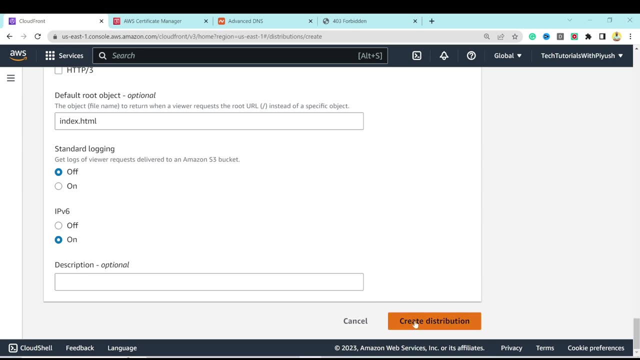 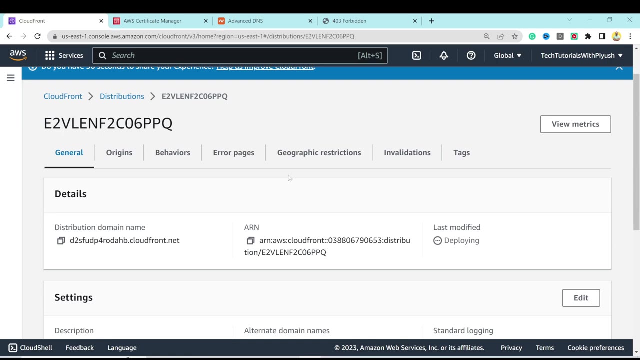 so it says we have to choose the firewall. so let's choose it and keep everything default. i guess this was something that introduced recently, because i didn't see this setting earlier anyways, so i have enabled it and hit create distribution. okay, now it's gonna take 10 to 15 minutes because it's gonna deploy the edge location in multiple. 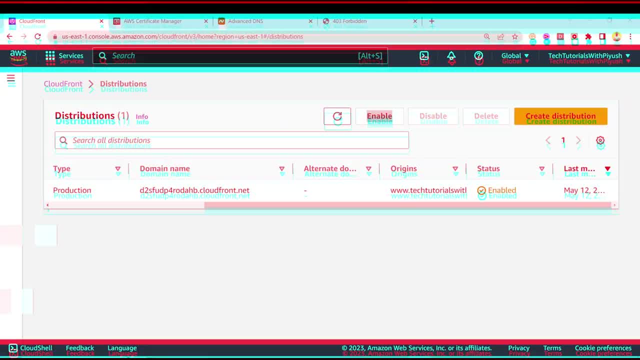 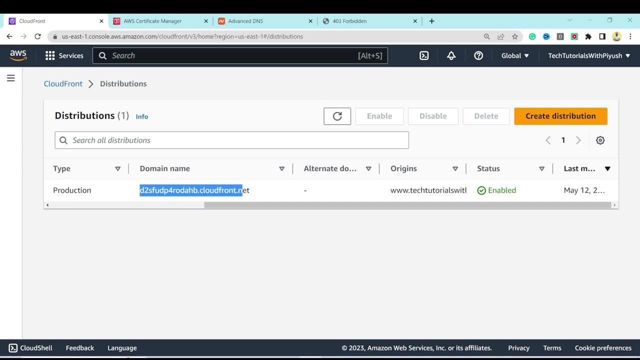 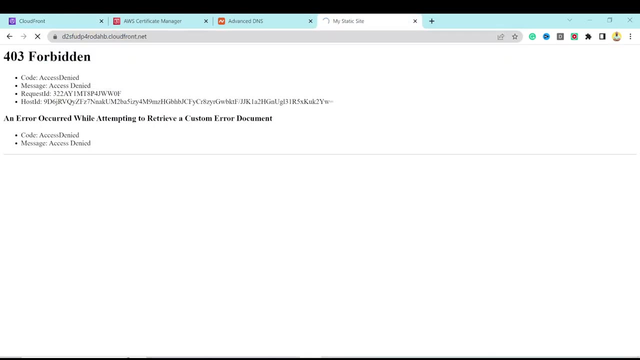 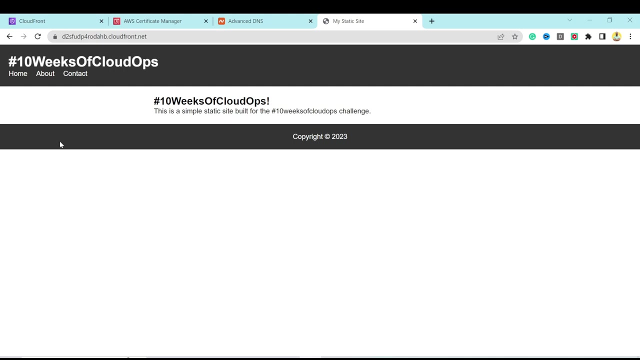 locations, so it's gonna take some time, so all right. so after five minutes or so now it's been deployed successfully. now our website should be accessible on this domain, which is the cloud front url. let me copy this and paste it in a new tab: and yes, it is there, and it is secured with https, and this is what we wanted to do. 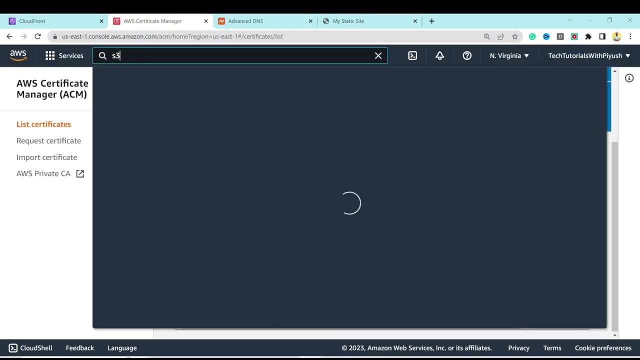 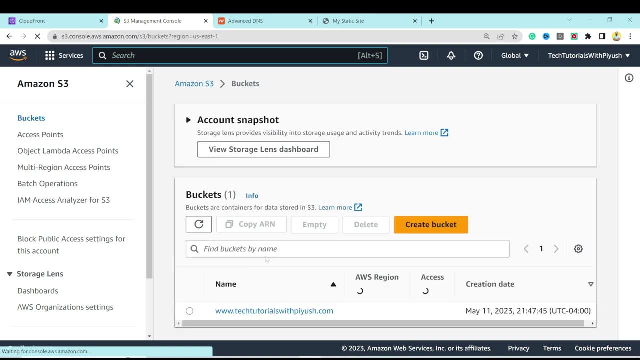 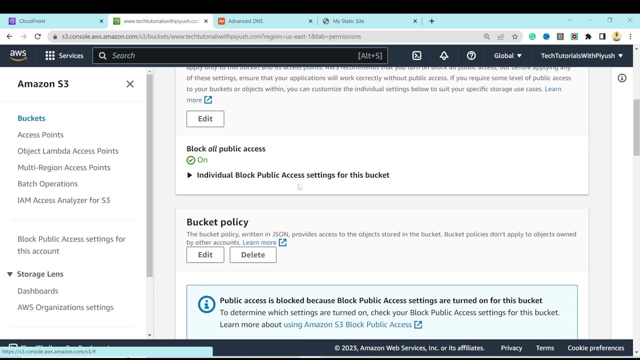 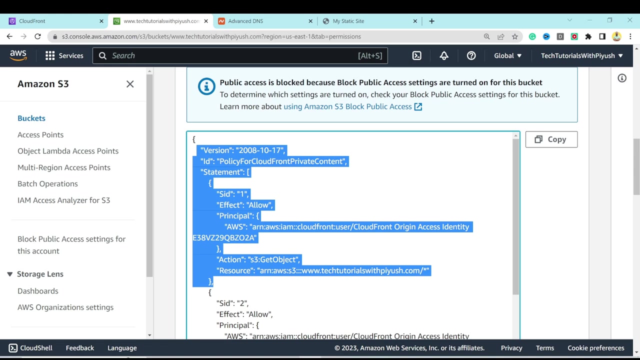 now let's go back to our aws console and go to s3 bucket. i'm going to show you one more thing. so go to the bucket and then go to permissions, scroll down a little bit and you will see a bucket policy created for you. we didn't create this policy, but it was created when we enabled the cloud front distribution. 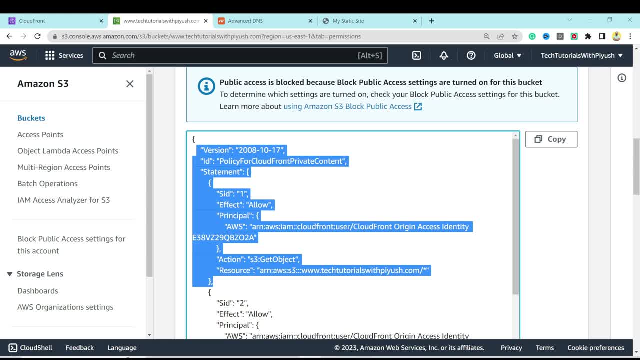 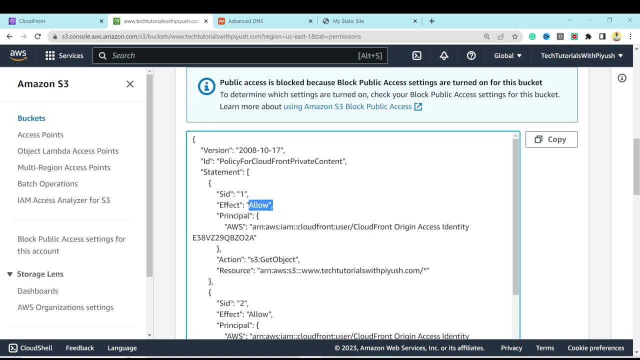 remember it says yes, update the bucket policy. there was an option there, so that option created this. what it is doing it? it is allowing the access from this cloud front origin access identity to s3 garage. if we have the domain name, it means we are going to have an object on this resource, which is our. 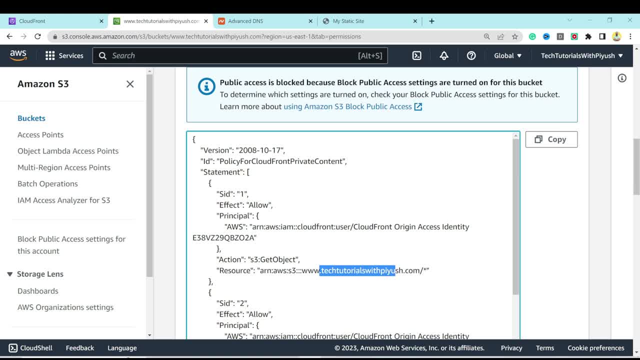 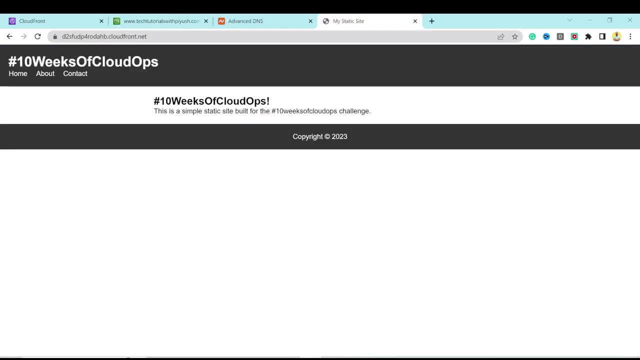 domain name, so that means the object inside the s3 bucket. this has three bucket will only be accessible from this cloud origin access identity. all right now, this website is hosted on our cloud front and this is not accessible through our s3 bucket, which is, we have already seen. 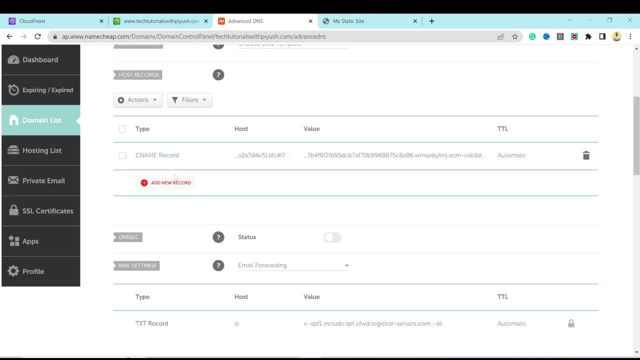 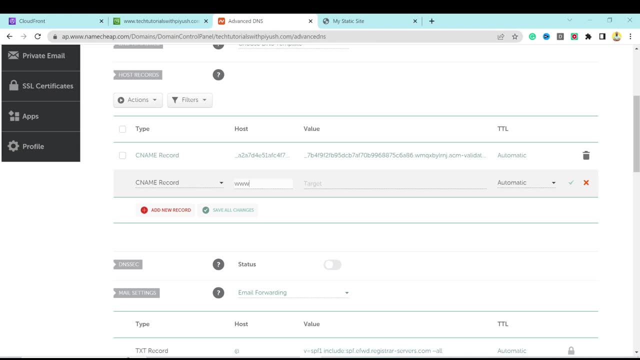 this from here and go to our namecheap. now i need to create two more cname records over here. let's go ahead. first, cname record: host should be www and target should be this: without a https, just the domain. remove it and hit save. okay, now add one more record. 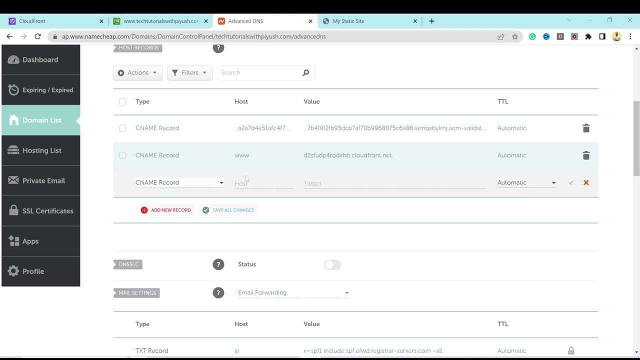 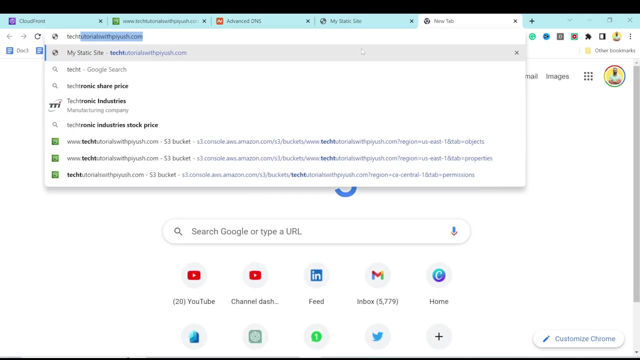 which will do the redirection, cname record and host name will be tech tutorials with pugecom, and target should be our cloud front distribution, please. okay, now go back to your web browser and go to tech tutorials with pugecom, which is my custom domain. hit enter and it will. 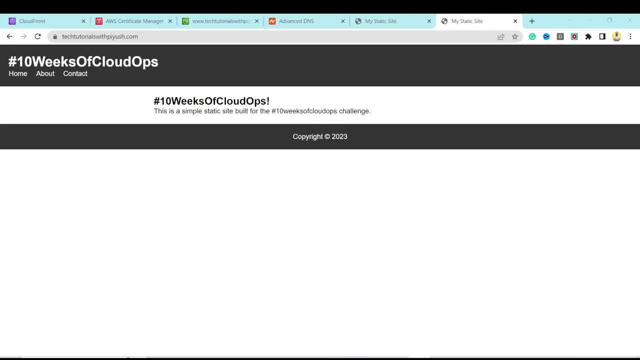 record. the cname record and host name will be tech tutorials with pugecom take a couple of minutes and after waiting for a few seconds, it worked. now my website is accessible on my custom domain. this is what we needed, so let's quickly see how we can automate. 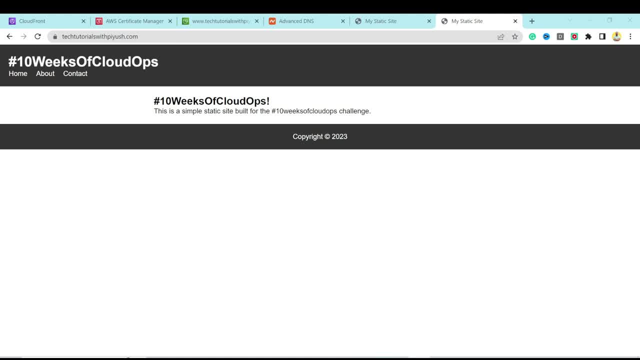 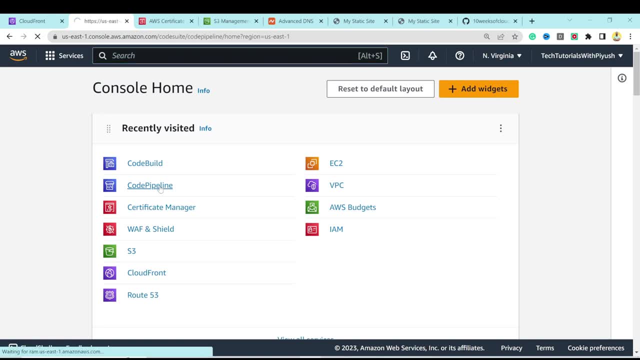 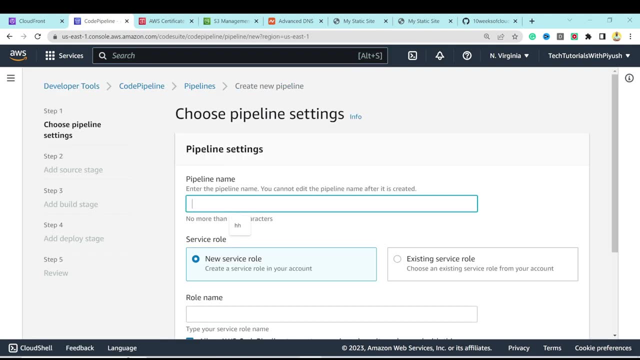 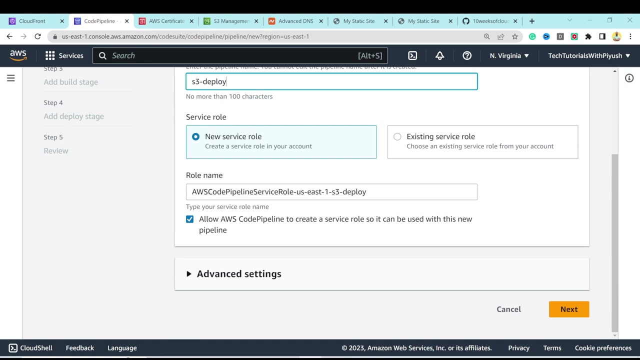 the ci cd using code pipeline. so now i'm gonna go ahead to my aws console and and look for code pipeline. then i need to create a new pipeline by hitting over here: create pipeline. give it a name. let's call it s3 deploy. now we need to create a new service role or if you have any existing, 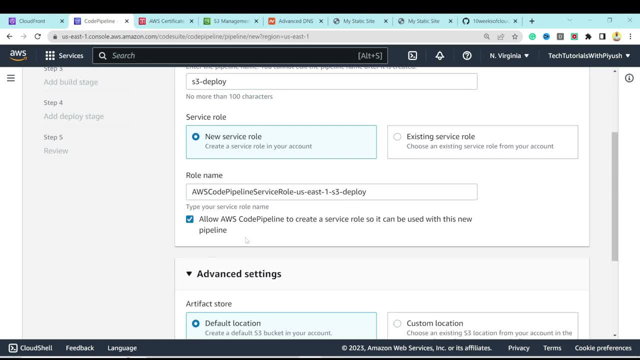 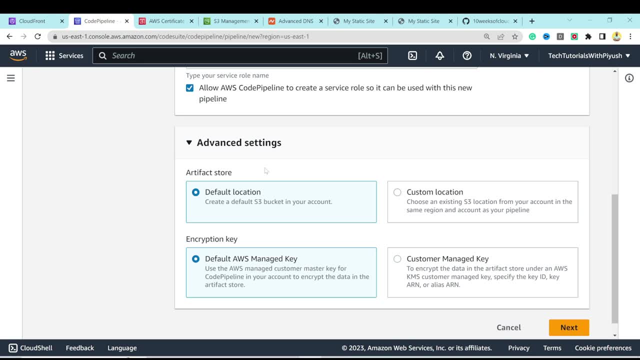 service role. feel free to use that advanced setting. it says artifact store. that means the static files that are part of this website will be stored in a location in an s3 bucket. you can use an existing bucket or create a new bucket, so this first option will create a new bucket for. 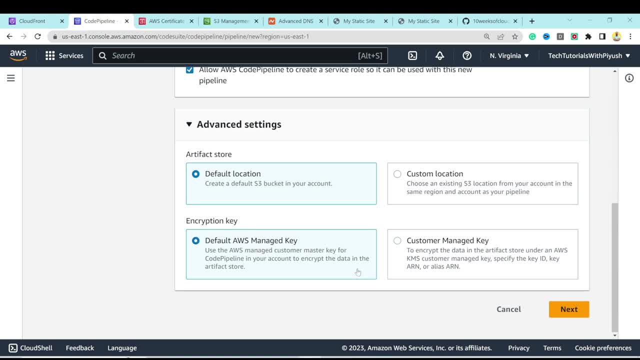 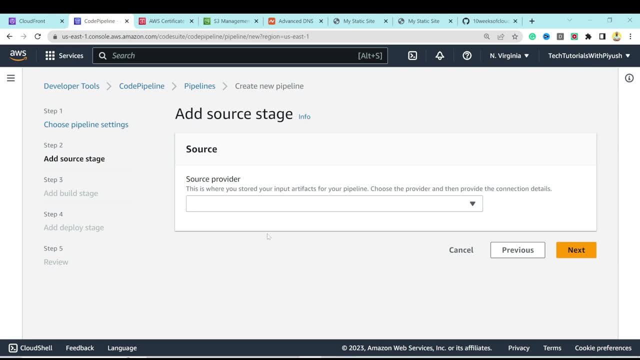 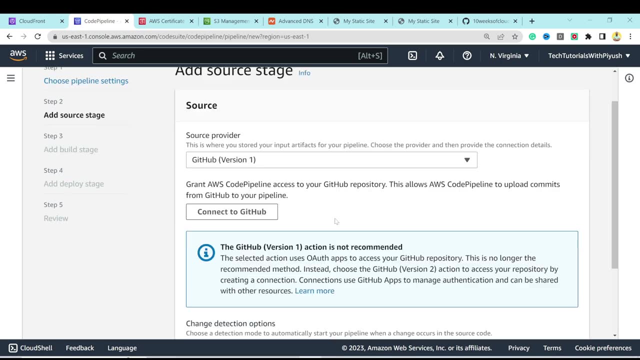 you and encryption option: let's go ahead and create a new bucket for you and encryption option: let's keep it default. click next now. source provider is where your files are located initially, so my files in. it isn't a github repo, so i'm gonna use github version one. now i need to make a connection with github. 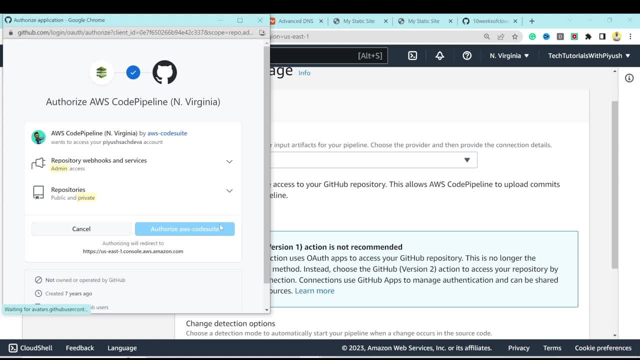 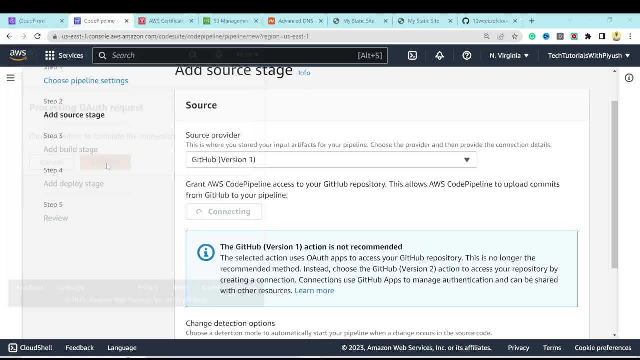 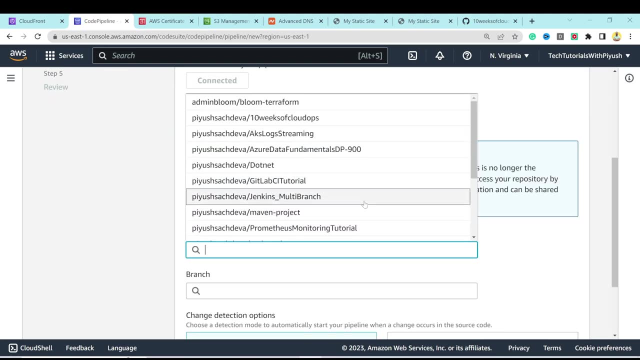 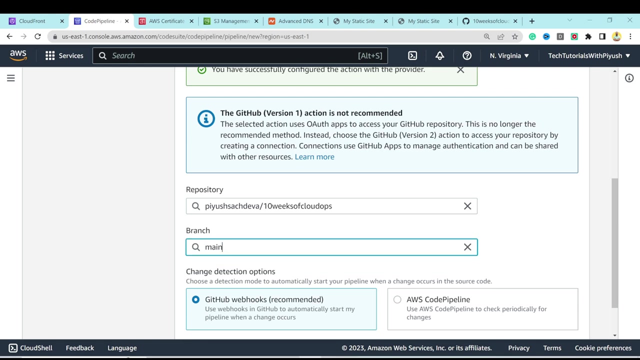 so hit over here, connect to github and authorize and confirm. that's it. you have successfully configured the action with the provider. now, if i see the drop down, i will see my repository over here and the branch is main. i only had one branch created. now the change detection would be github. 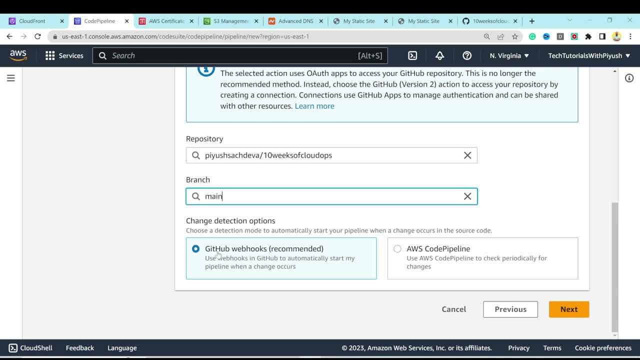 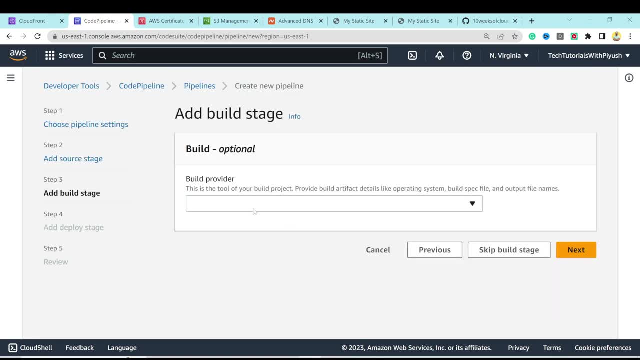 webhook. that means whenever there is a change in the file, it will trigger the pipeline and deploy the new files to the s3 bucket. now build provider. i don't get the name of the provider and i don't really have any build process over here, because those are just the static files, so i'm gonna skip. 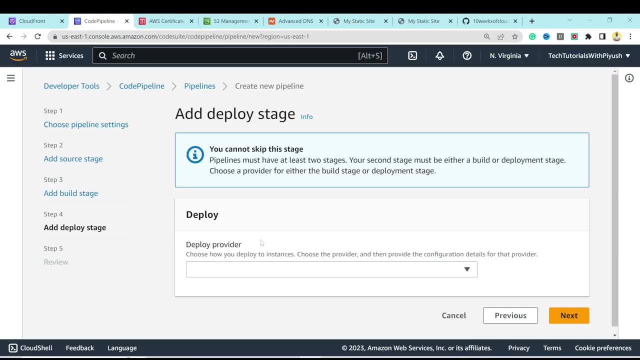 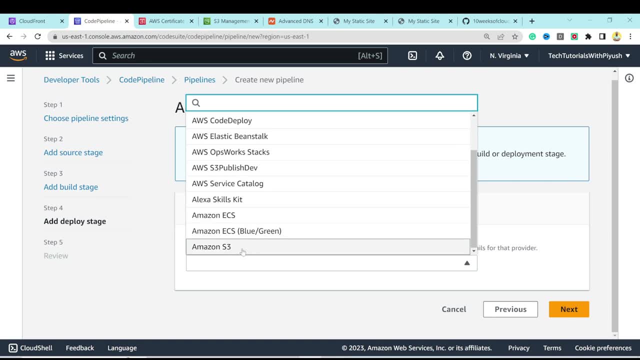 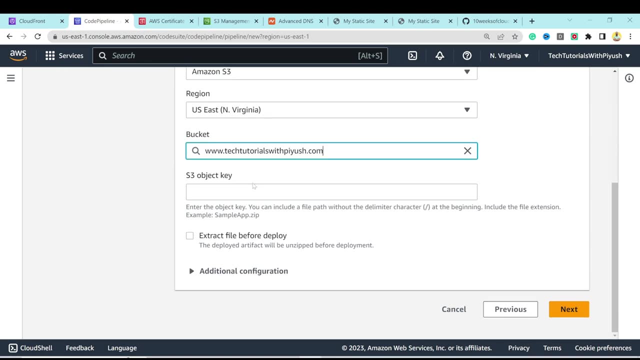 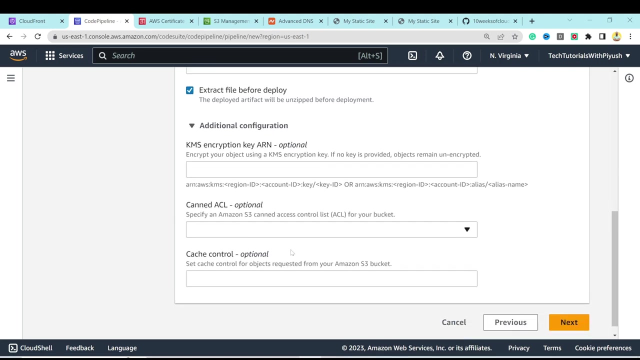 the build stage, right skip. now the deploy provider should be s3, so let's go ahead and select amazon s3, the bucket is this one: my custom website. s3 object key. then extract file before deploy and let's see if it has any additional configuration. that's it hit next. 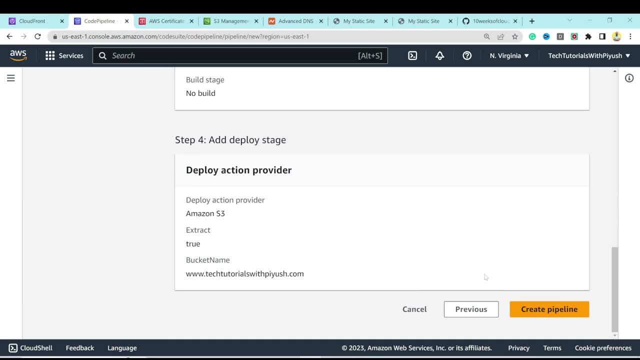 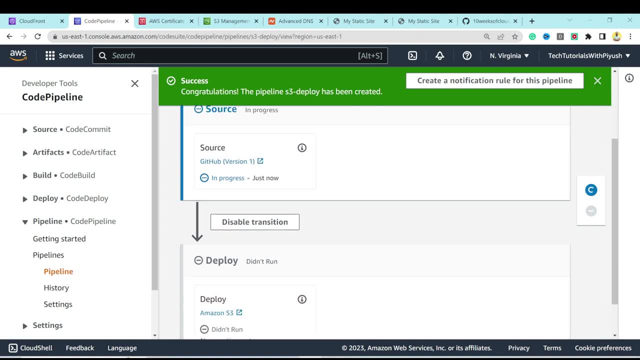 and review everything and then create a pipeline. now it triggered the pipeline for you. let's see: the git checkout is in progress, succeeded and it deployed the file. now how do we know that it is completed successfully? so let me go ahead to my github repo and make some changes. 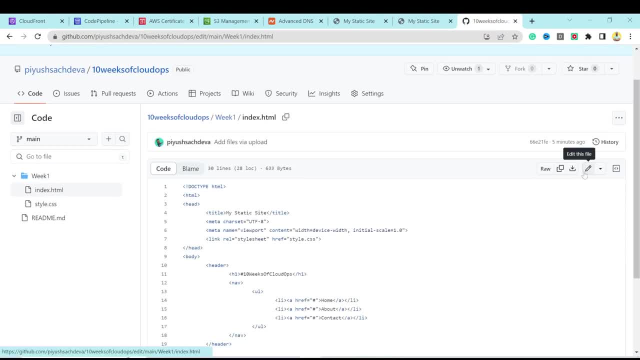 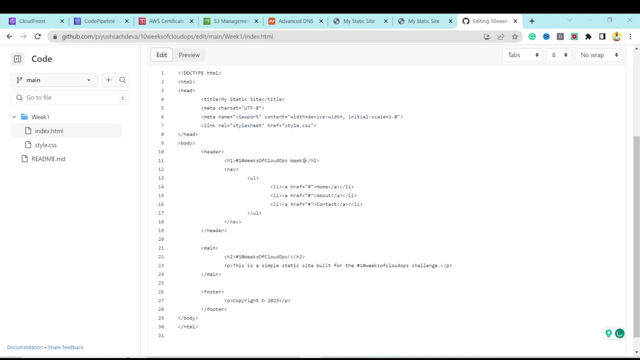 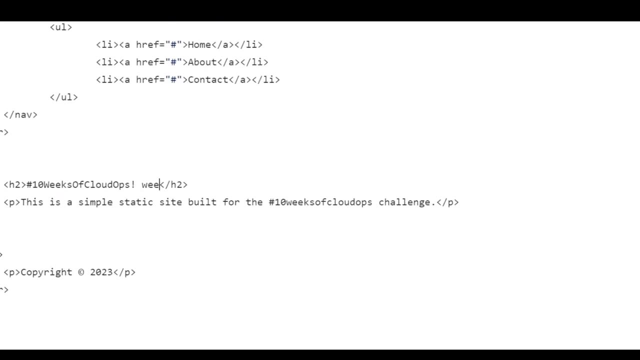 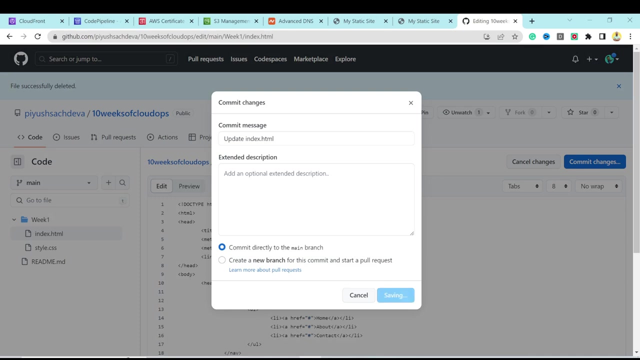 so let's go ahead and create a pipeline and let's see if it has any additional configuration. go to indexhtml, edit the file and let's make the changes over here. call it one over here as well. one, commit the changes and now it should auto trigger the pipeline because we have just 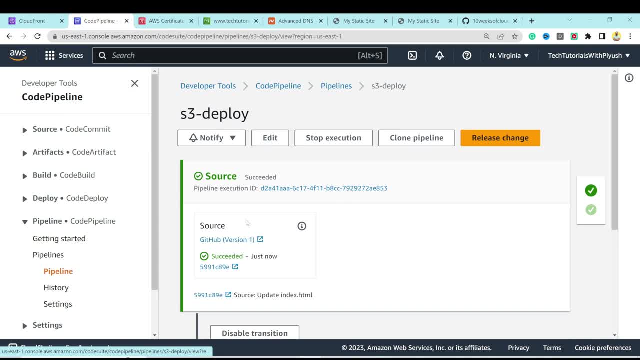 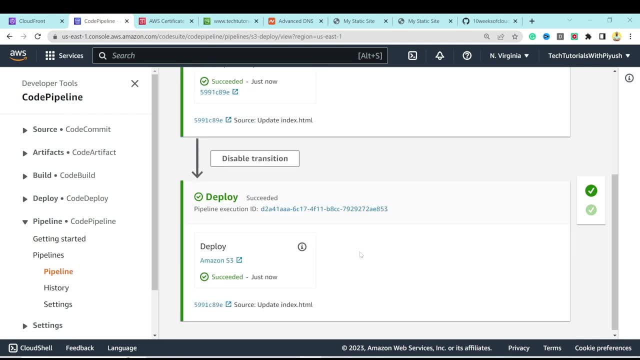 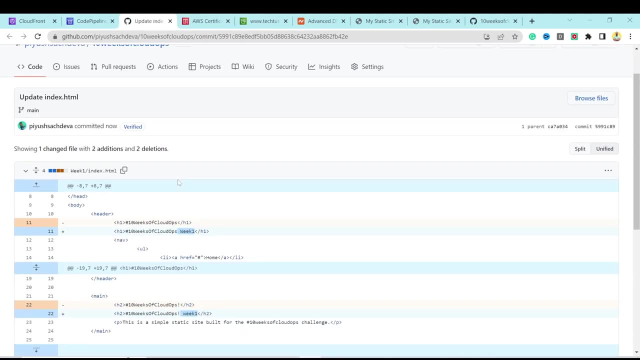 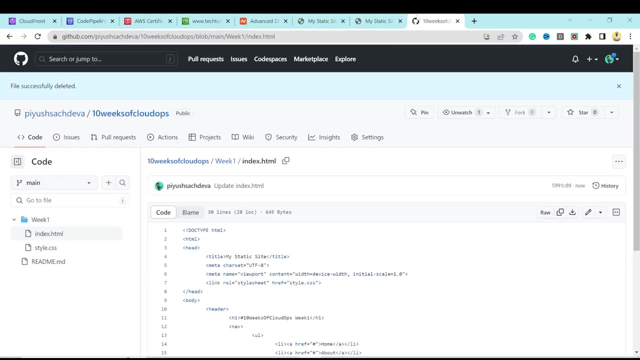 committed the changes. let's see go to pipeline. this was the older version. oh, it just got completed and the source was update indexhtml and it detected the change as well. like this was a change that we just made, so now let's go ahead and hit refresh on website changes, is not there? the reason for that is: 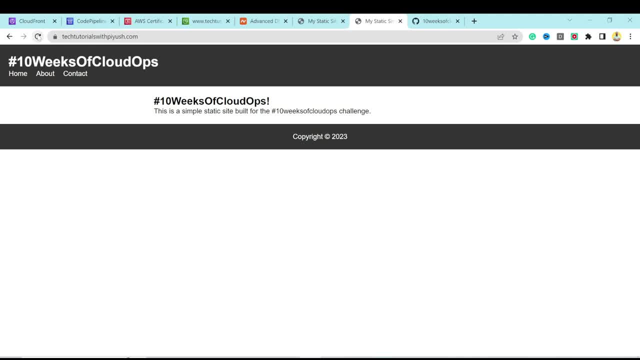 because cloud front caches the static content in its edge location for some time, right once the cache is invalidated or paused. only then we will be able to see our refreshed content. if we were using any other ci cd tool, then we could have added that invalidate cache option in that. but 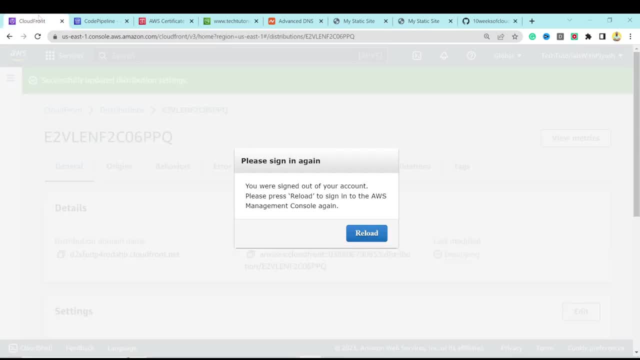 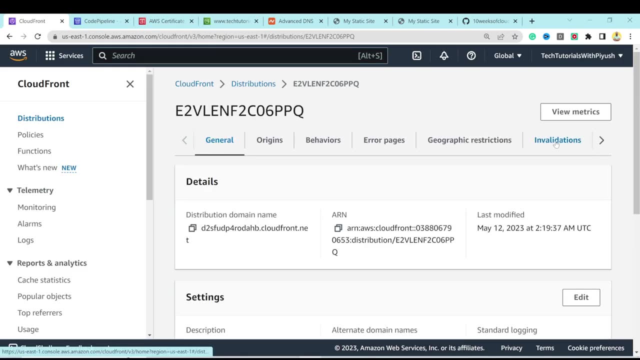 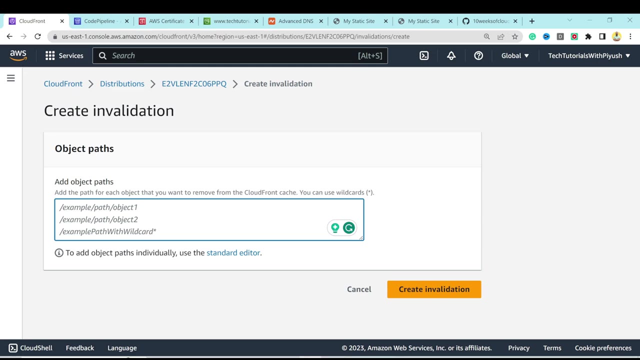 aws code pipeline doesn't have this option. so what we can do is we can go to cloudfront and invalidate the cache manually. so go to cloud front and then hit over here invalidation, create an invalidation, and over here we need to give the path. so let's do wildcard for all the files. hit create invalidation. 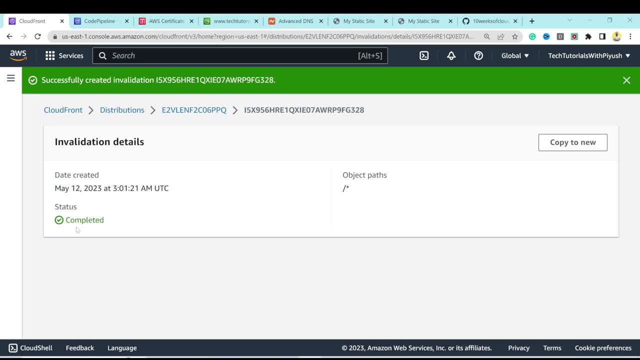 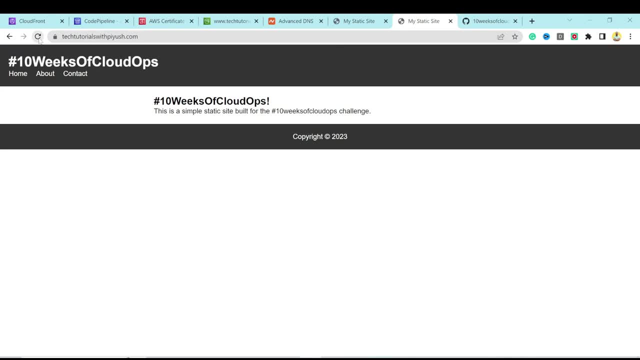 okay, it says completed, so ideally, our content should be refreshed now. so let's go back to our website and hit refresh. i still don't see the content, so i still don't see my content. maybe something is wrong with the s3. let's go ahead and. 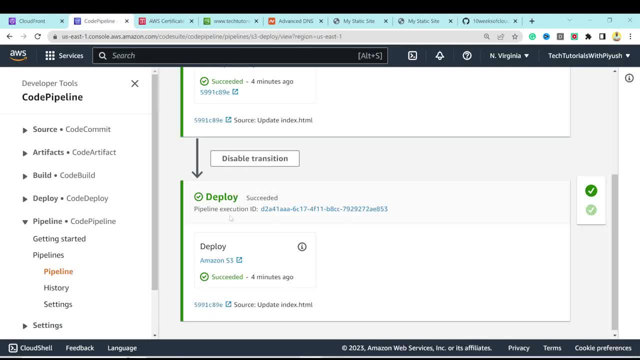 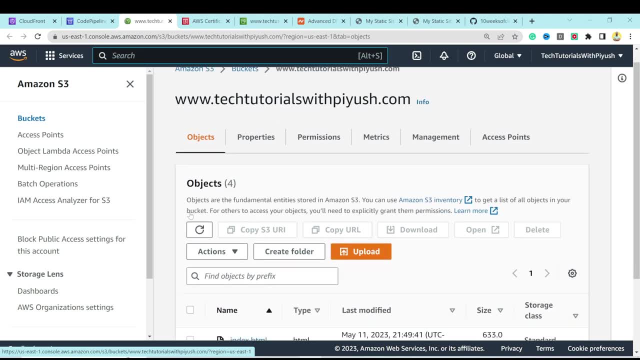 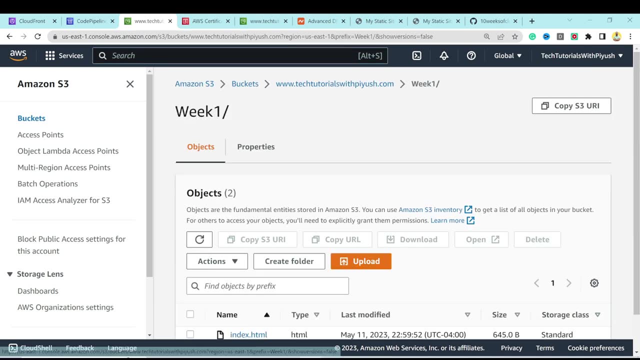 have a look at the code pipeline. so let's go to our s3 bucket and see if our updated file is there or not. okay, that's why. because, uh, in github repository we have this folder week one, in which there are two files, but as part of our upload that we did,